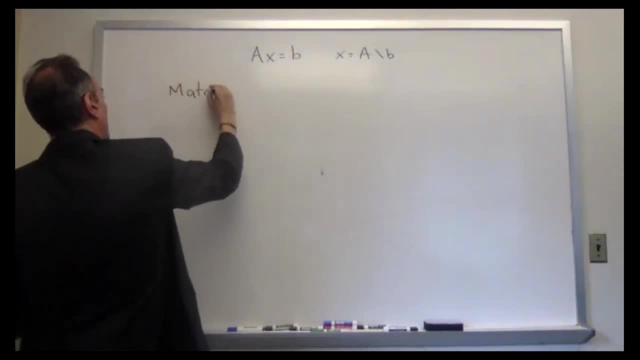 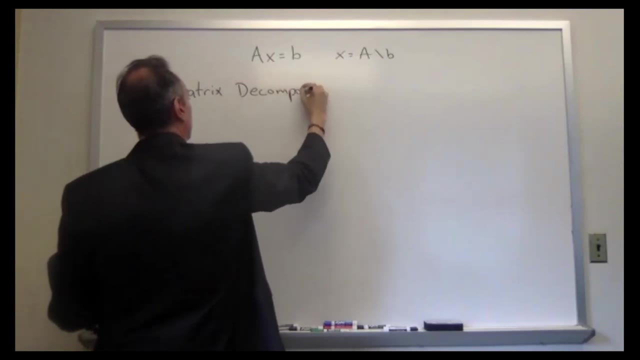 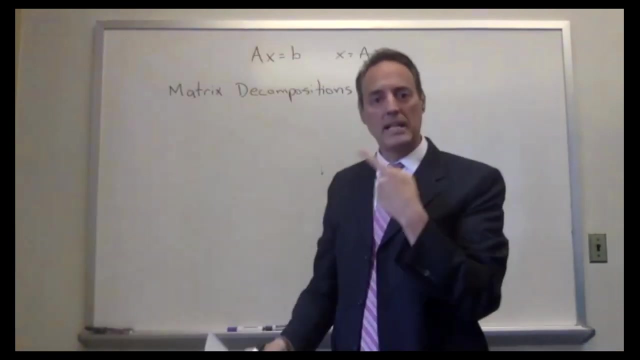 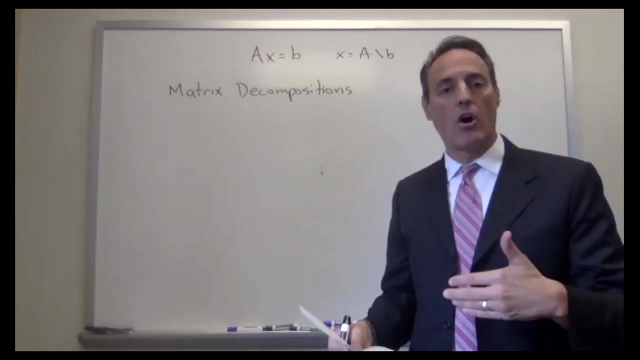 And what I want to do through the quarter is go through all these different matrix decompositions. So what is a matrix decomposition? Well, it's to take that matrix A and potentially write it in a simpler form so that we can solve X equal to B much more rapidly. 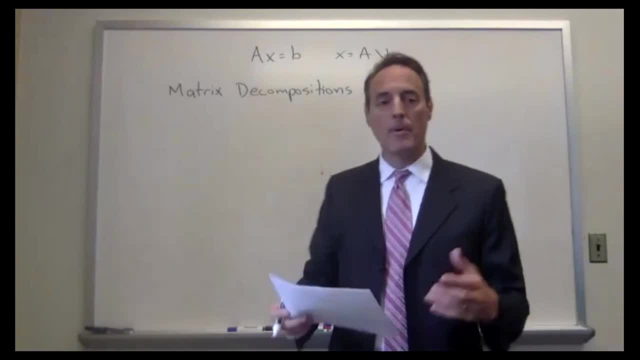 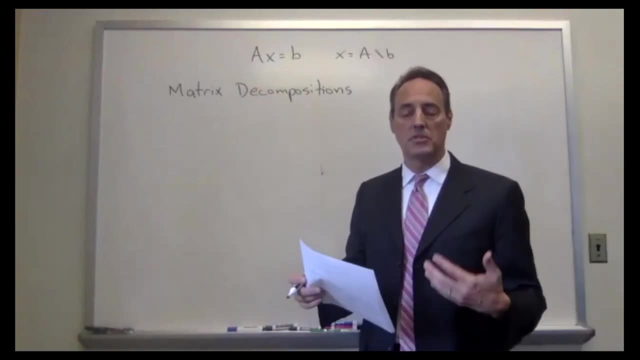 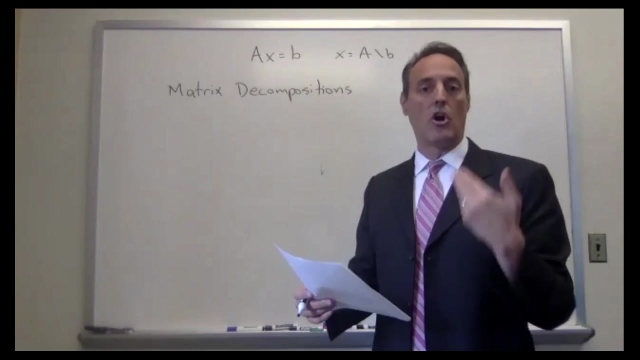 Okay, So I'm going to list over here a number of matrix decomposition techniques, And what I'm going to show you is that with these matrix decomposition techniques, there are lots of uh advantages- if you can decompose this matrix to solve the problem faster. 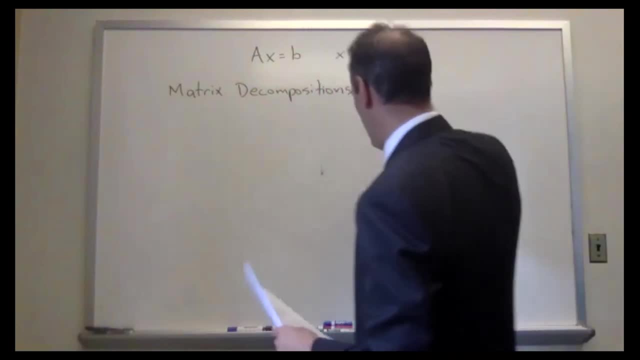 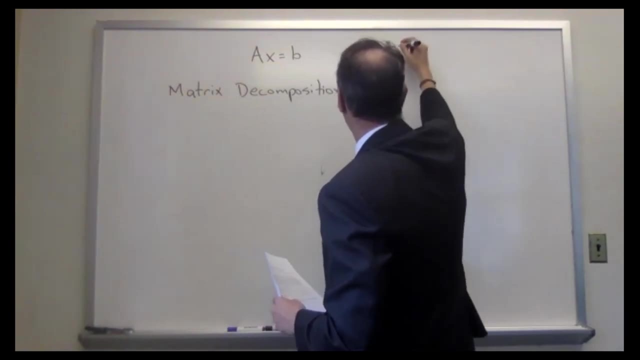 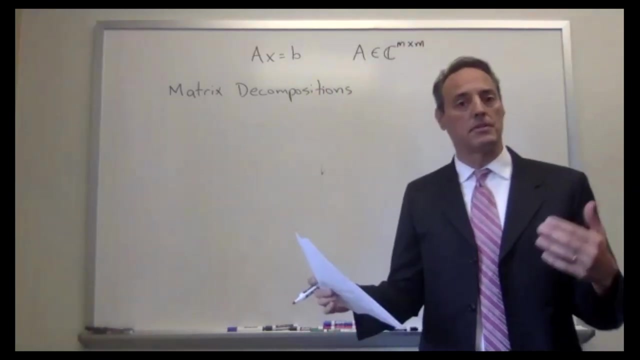 Initially, let's start off with matrices A, And they can be complex numbers that are m by m's. Okay, they're square matrices. We're going to relax this in a bit. We're going to have to talk about what it means to have a non-square matrix. 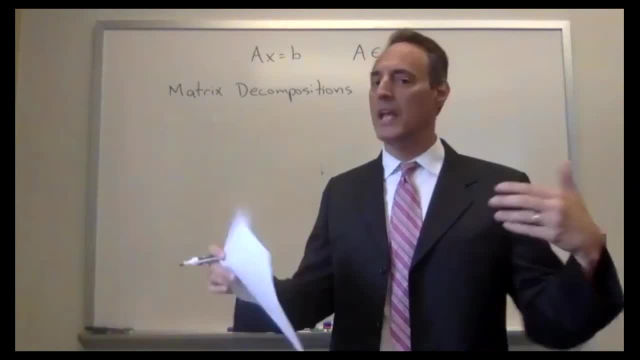 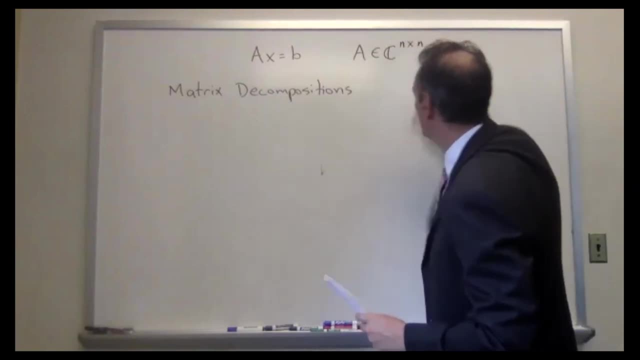 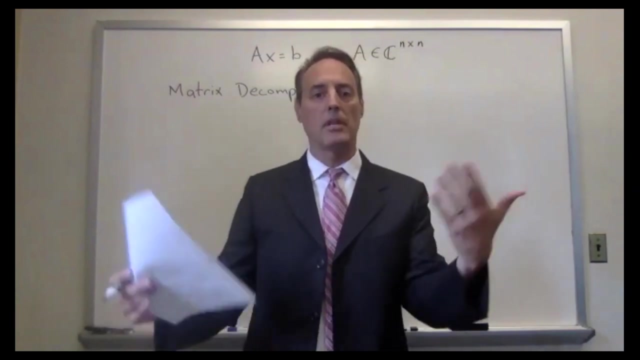 In a little bit, But right now let's just assume I have m equations and okay, let's do n by m, not m by m. Okay, n equations and unknowns. And this is what you probably had in linear algebra And you figured out how to solve this, And typically the way we did this in linear algebra was to do Gaussian elimination. 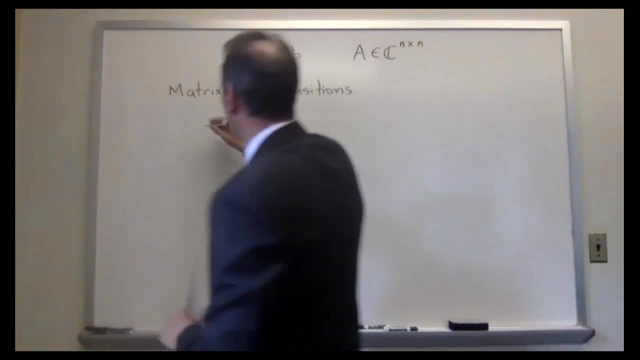 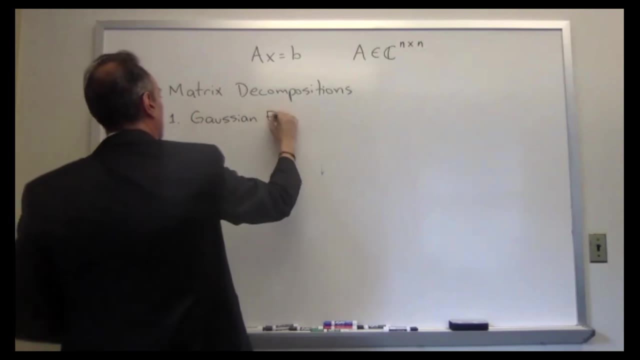 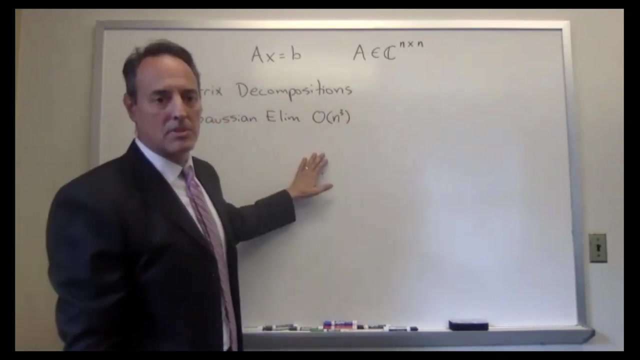 And Gaussian elimination to solve this. I'm going to put this here: It's not a decomposition. Okay, It's going to cost you around. you can be more precise than this, but it's going to cost you around. order n- cubed operations. 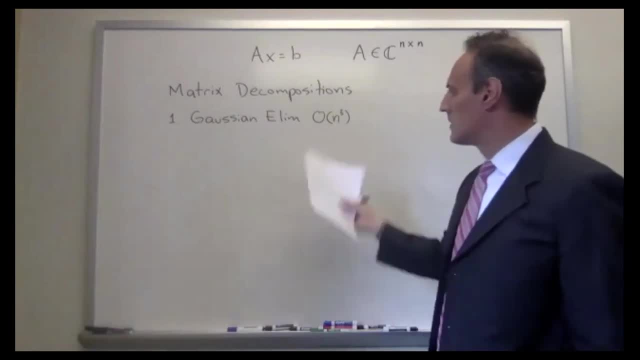 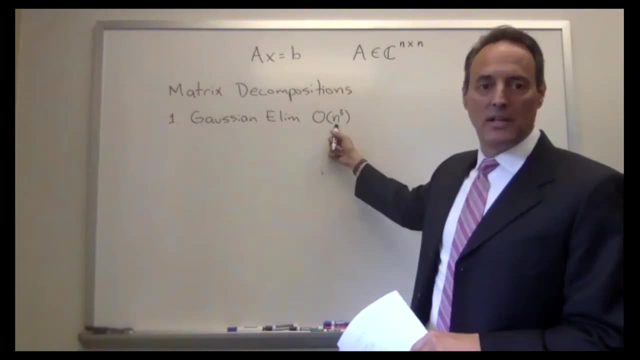 Okay, So if it's a small matrix, that's not a big deal, But part of what we want to do is go to big matrices, And you can see as you go to big matrices, you're cubing this thing. So this is problematic. 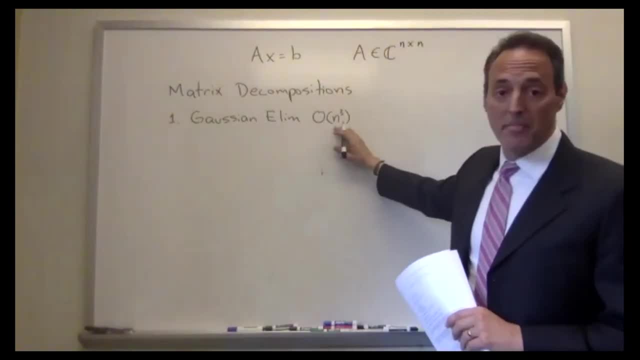 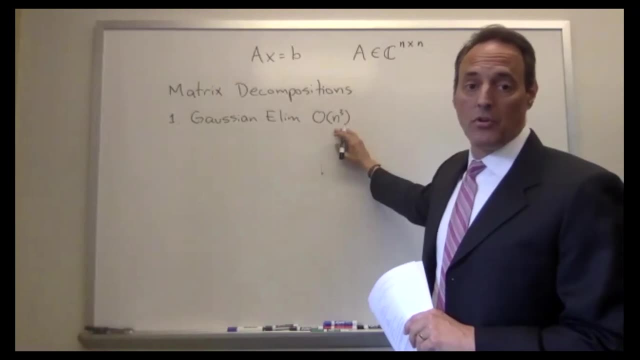 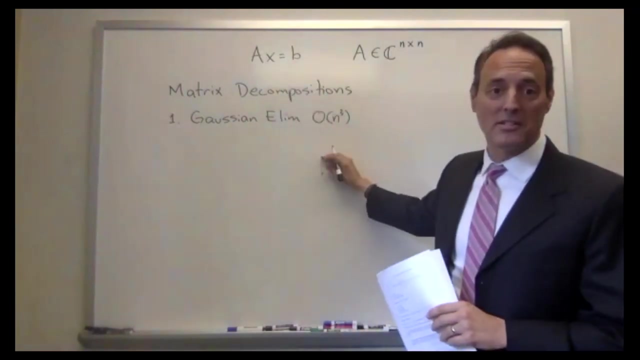 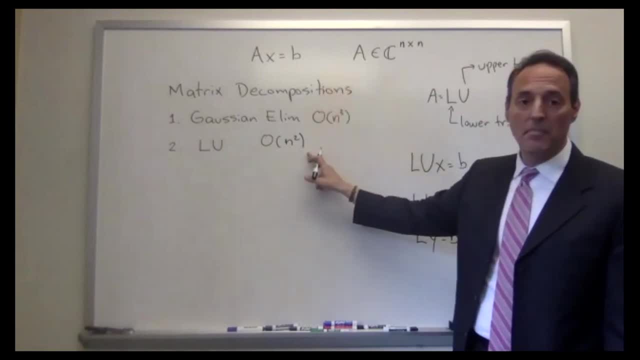 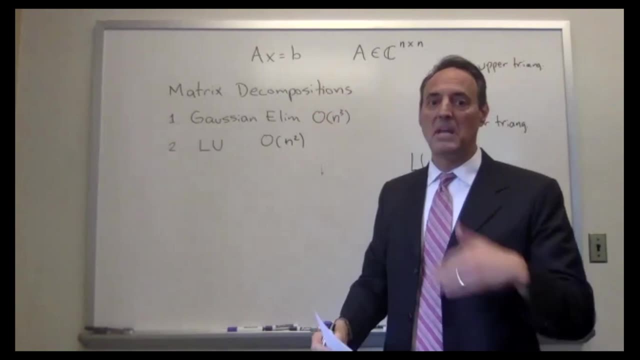 You can see the problem. If you're doing this in data analysis, you're going to get 10 to the 27.. a thousand matrix: this is gonna be a thousand times faster, right? these are the kind of speed ups you're looking for in computation. it's these speed ups in computation that have allowed us to. 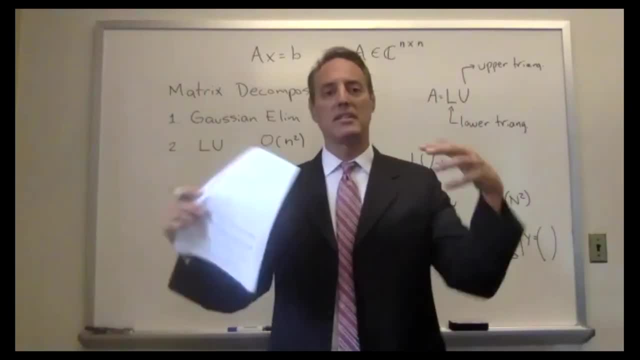 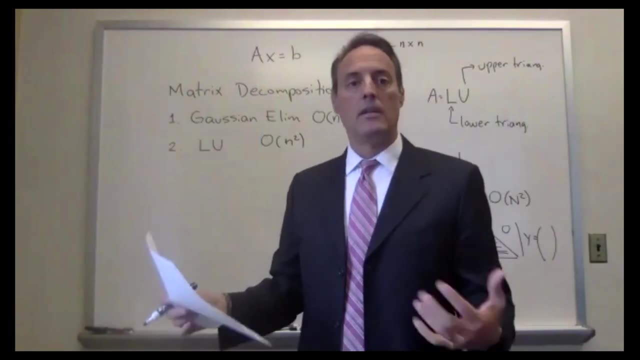 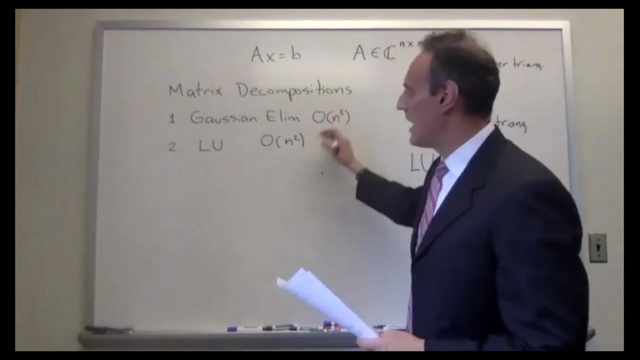 solve some of the grand challenge engineering and science problems of the day, like basically modeling airflow over an entire airplane, you need fast computation algorithms. these are the kind of things that you're using. okay, so the lu has this advantage. the question is, how did you get that lu? 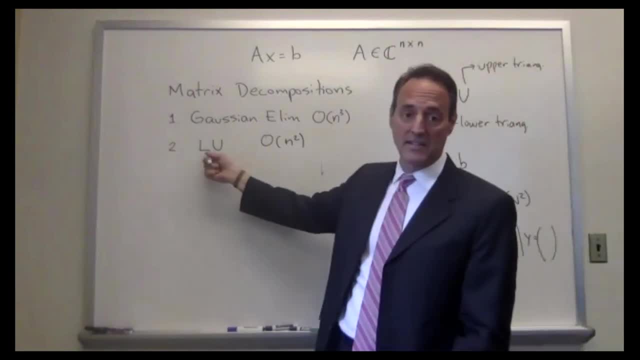 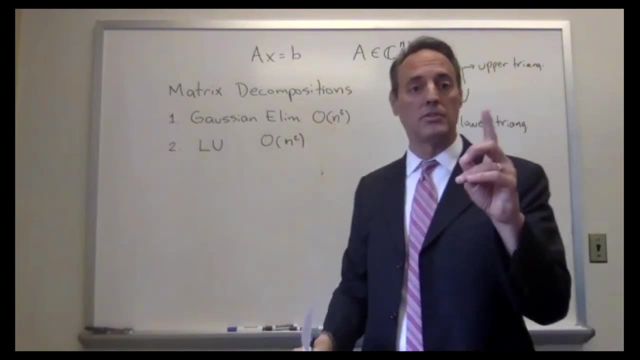 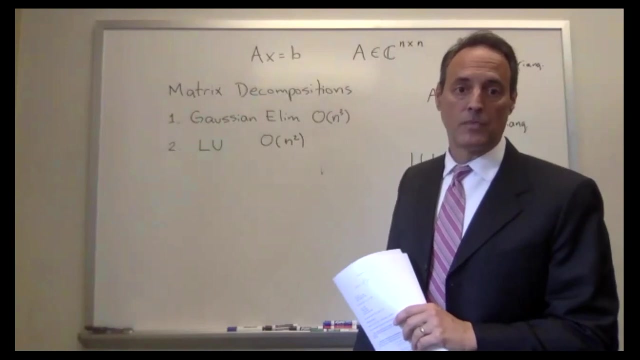 so we're gonna have to start talking about the cost of actually getting that. it turns out doing an lu. decomposition costs. you order n cubed, but you only have to do it once, because once you have the matrix factored you can use it over and over and over again for different b values. okay. 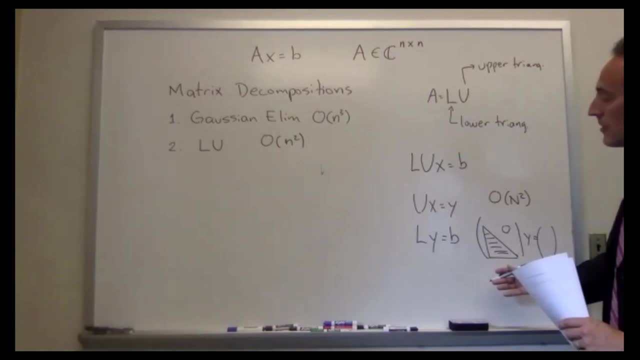 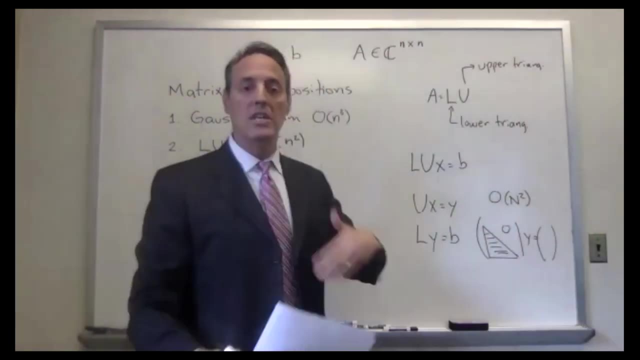 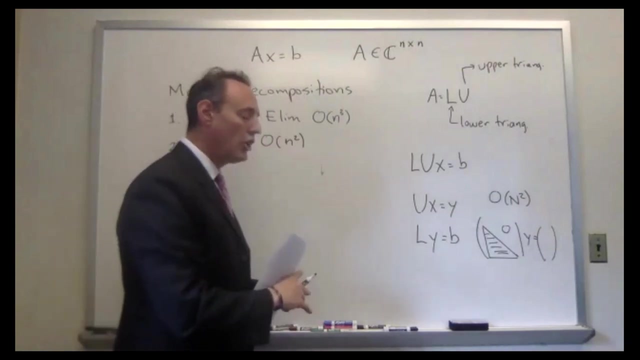 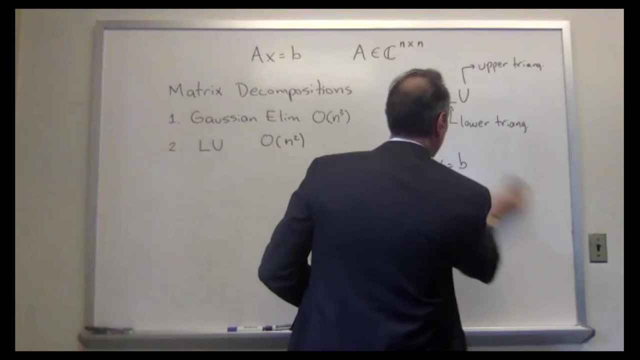 all right, so that's an lu decomposition. hopefully this makes sense of why you would use it, because once you have it, all you have to do is forward or back substitute. so this is a classic matrix decompositions- okay, used heavily in scientific computing. all right, that's one matrix decomposition. 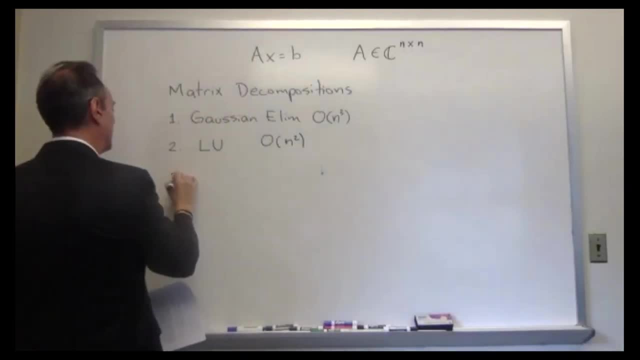 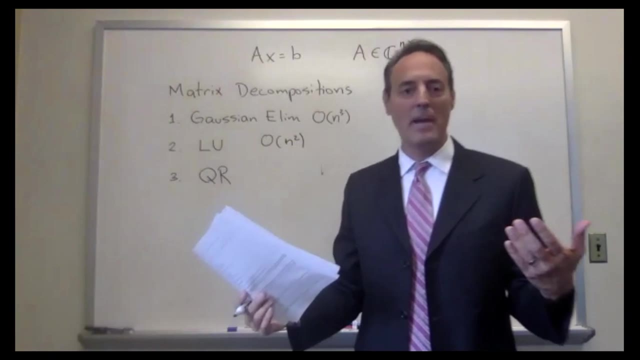 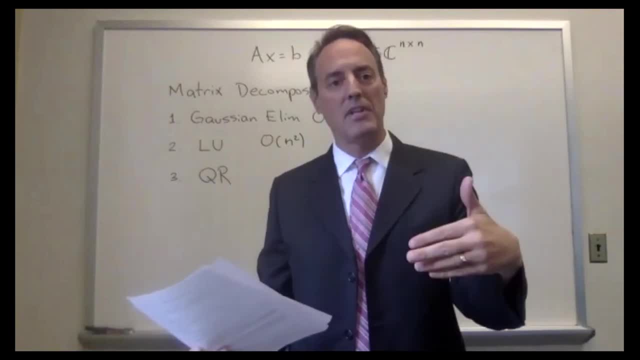 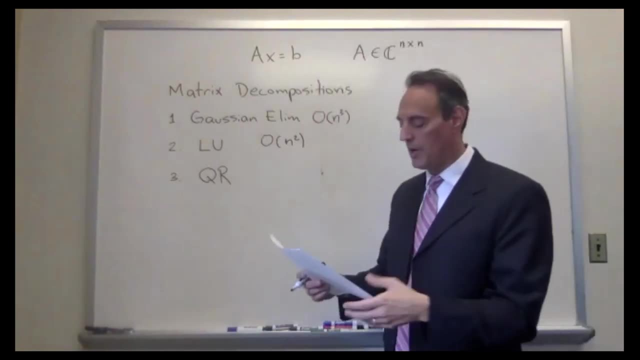 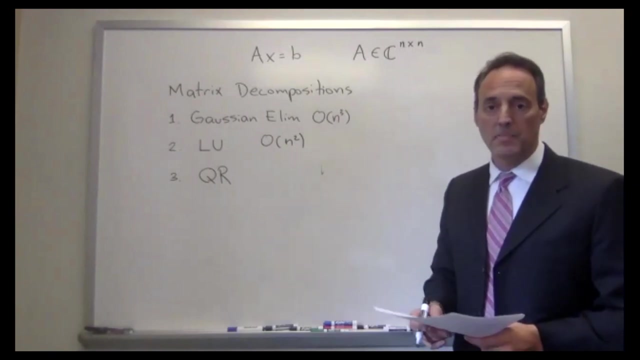 many is that people have tried lots of methods to get this thing to work okay or to try to improve speed. what are the kind of decompositions you come up with? qr, the qr algorithm, and we're going to spend quite a bit of time on qr in two weeks time. 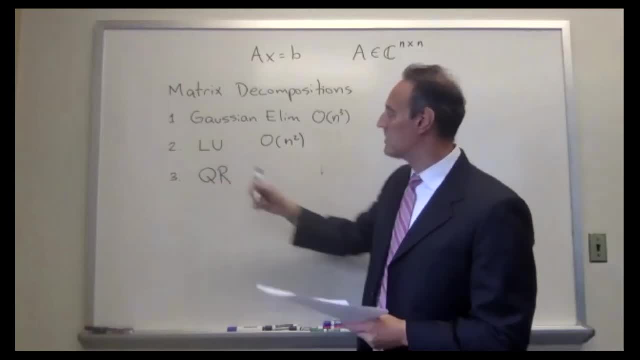 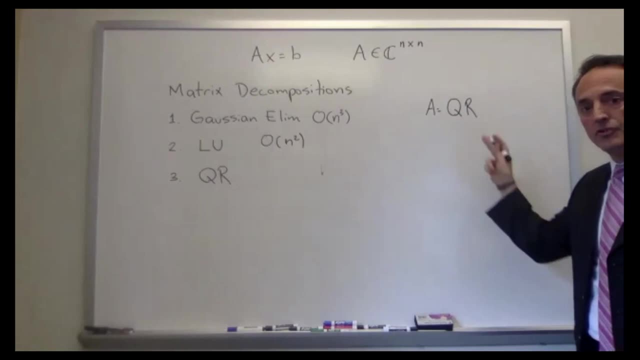 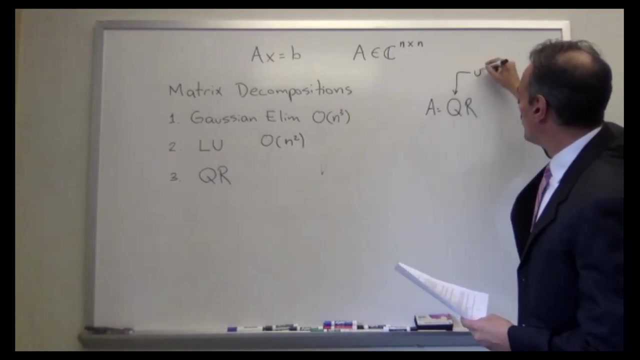 what this is is very much like lu right i'm. i'm going to take a and write it as a product of two matrices: q and r. now, what q and r are is: q is a unitary matrix. now, what's awesome about unitary matrices? and? 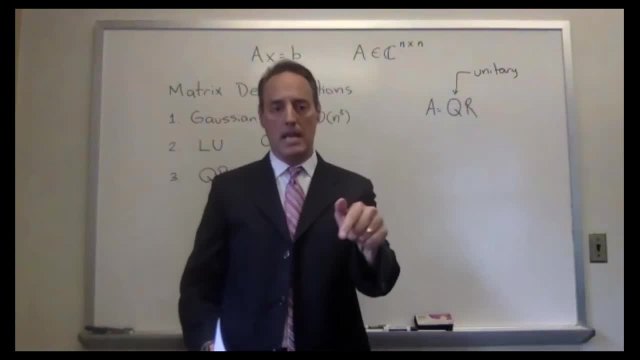 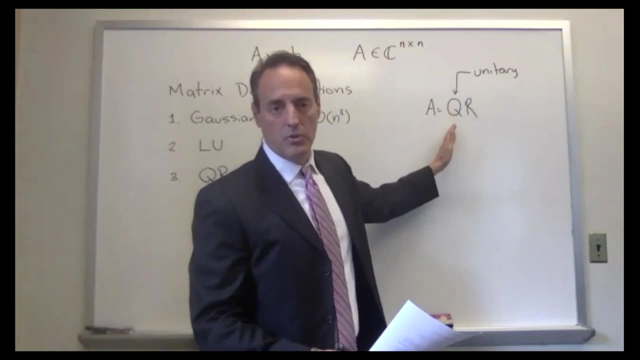 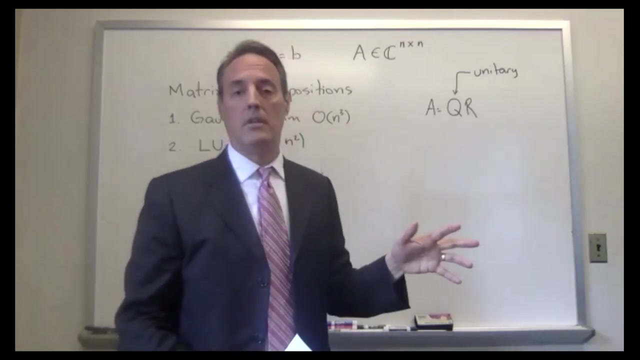 we'll talk quite a bit about special matrices on monday. unitary matrices, have it are such that the columns are orthogonal to each other and their unit length. so what's great about these matrices? the inverse is simply the transpose, transpose, complex conjugate. you're done, because usually computing an inverse of a matrix is is a very computationally. 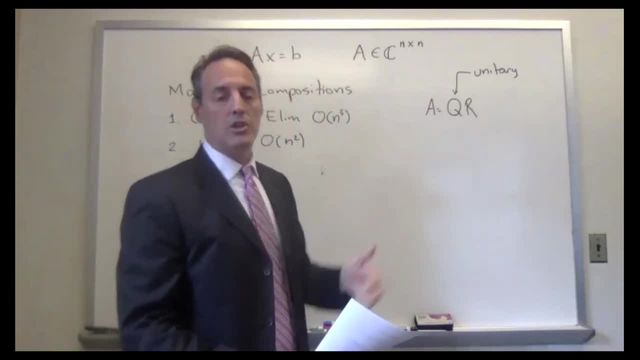 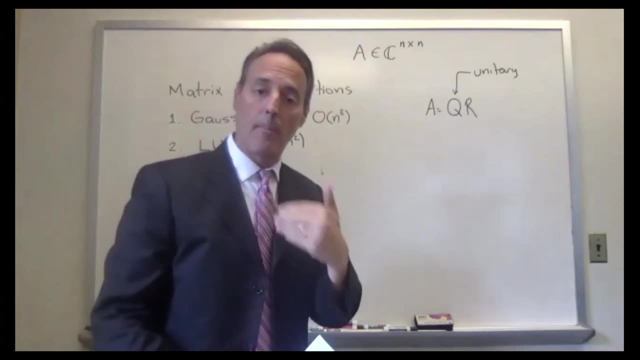 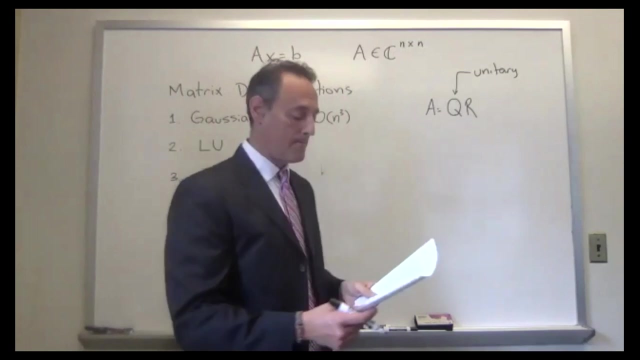 intensive here. it's trivial, okay. so there's really nice properties around unitary matrices and we're wanting to use as much of the properties as we can, of what these decompositions give us to take advantage of, of solving this. for these solutions, the r is upper triangular. 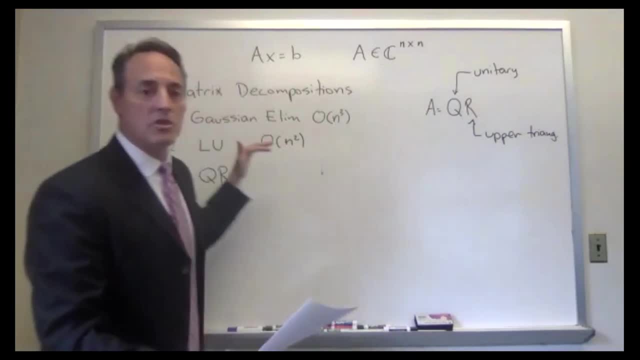 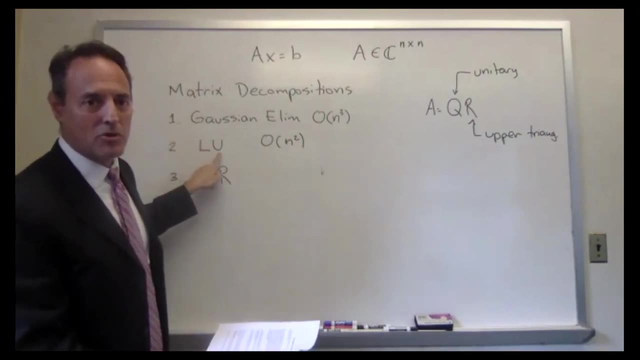 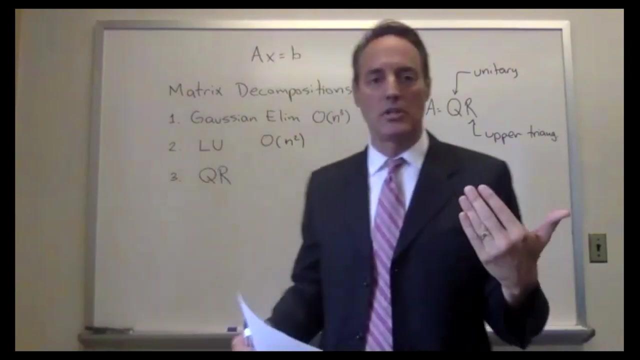 okay. so notice, interesting, when we do these deep different decomposition techniques like l, u, upper they, they represent u as an upper triangular, l is a lower triangular when you go to qr, r is upper triangular. so they're not consistent in their terminology. but just, that's okay. every decomposition sometimes calls me saying: 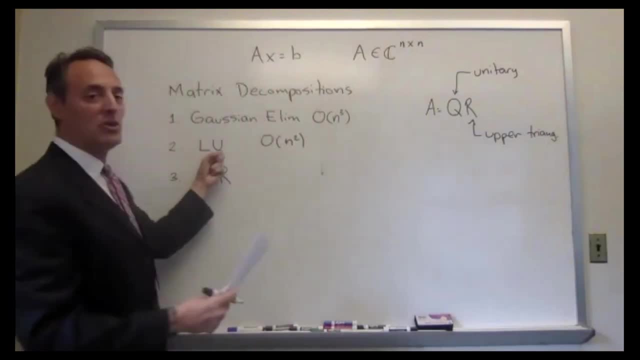 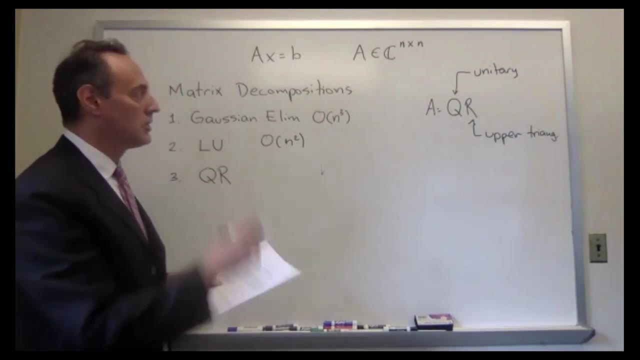 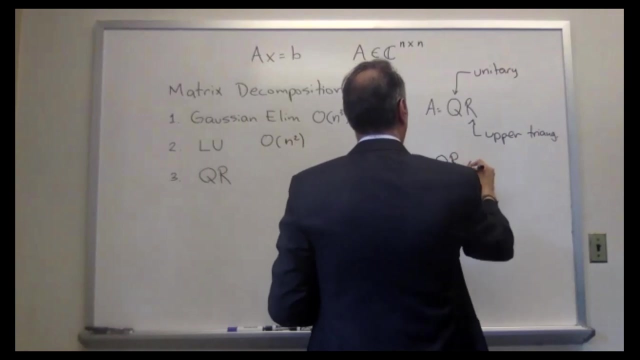 something different. just keep in mind that when you see a u, it doesn't mean it's always upper triangular, because in qr it's the r that's a triangular. so let's talk about solving the u and un ax equal to b with this. So now you have qrx is equal to b. We'll do something. 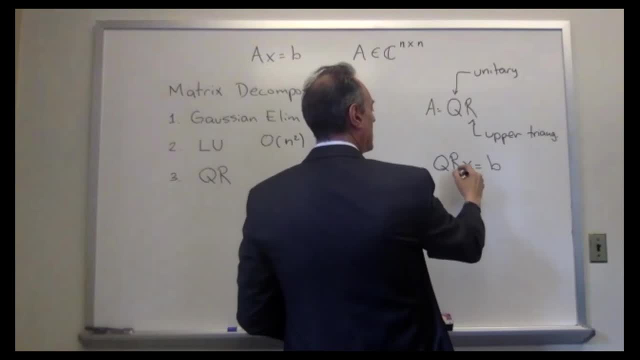 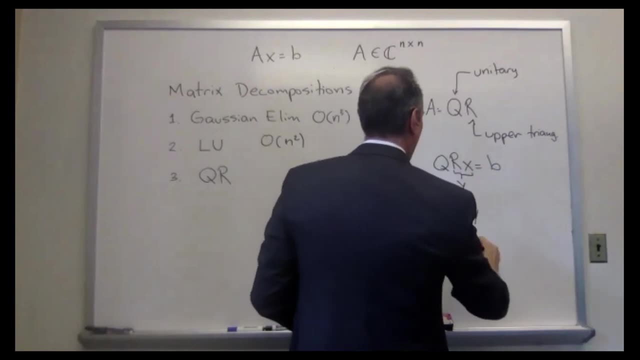 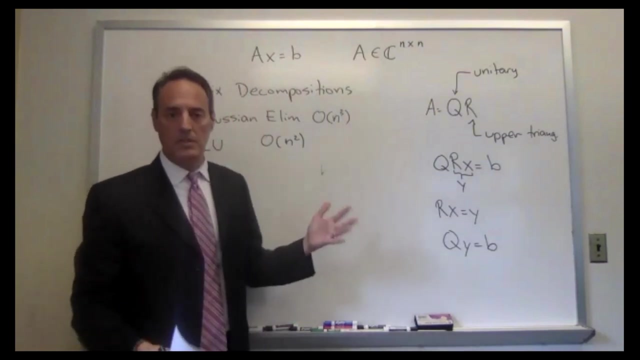 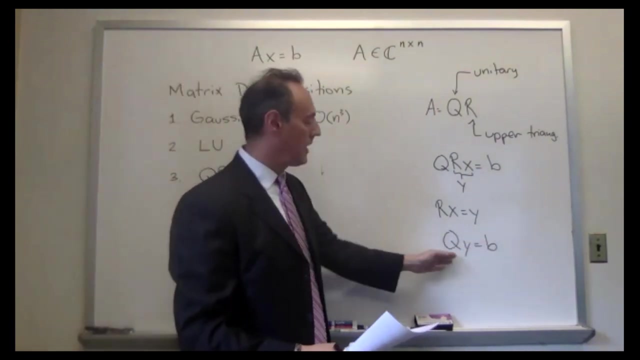 similar to what we did before. We'll call rx- y, So what you have is rx is equal to y, and then you have qy is equal to b. Okay, so it looks very similar to what we just did with Lu, but there is a big difference. When I go in here if I want to get the solution, 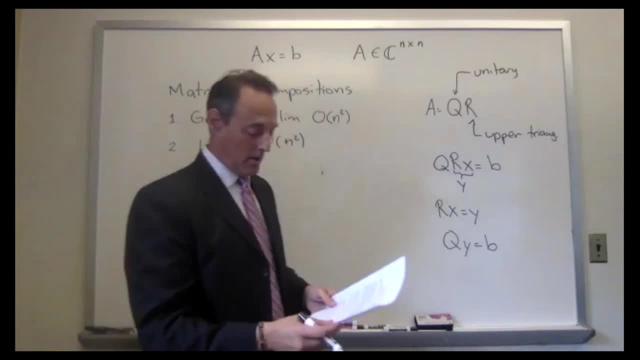 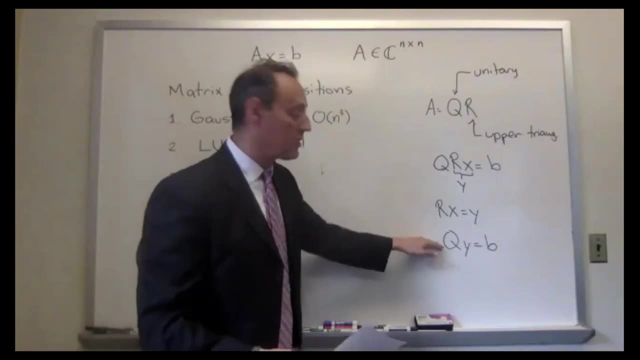 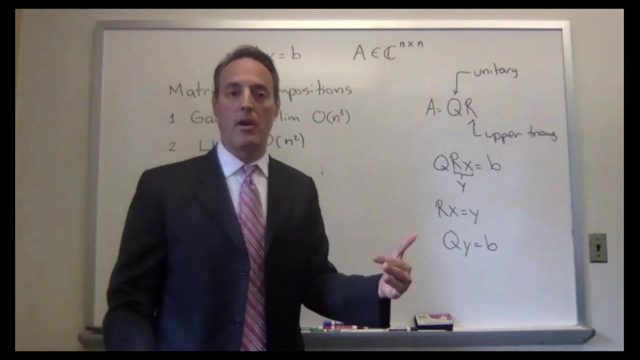 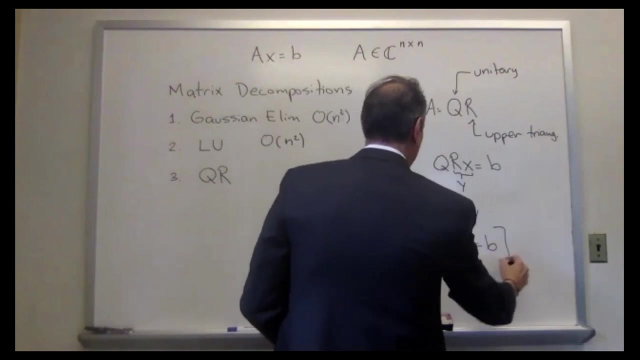 to y. all I have to do right is multiply now by q, transpose q. transpose q, because it's unitary, is the identity. That's the fantastic part of having unitary matrices. So if I take q, transpose on both sides of this, saying q transpose times, q is just the identity. so you get y. 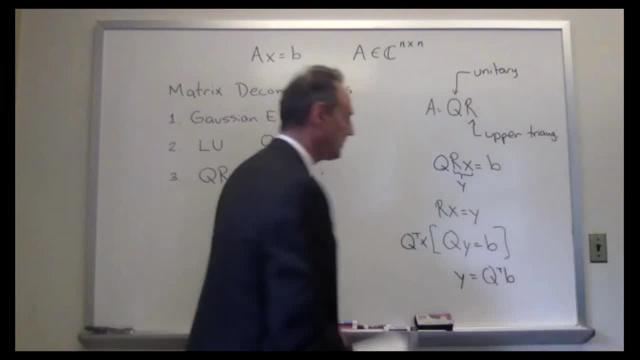 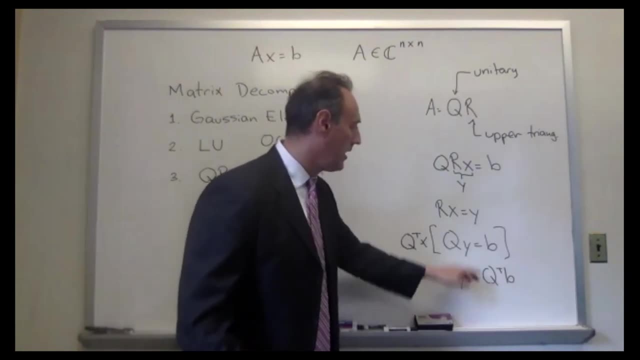 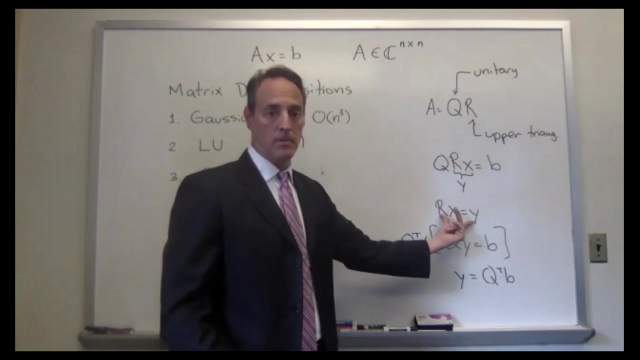 is equal to q, transpose b. so once i have this q matrix, all i got to do hit it with b to get y, bring it into here and that's upper triangular. so all i just have to do is back substitution. okay, so to solve the ax equal to b, i do one matrix, full multiply and back. 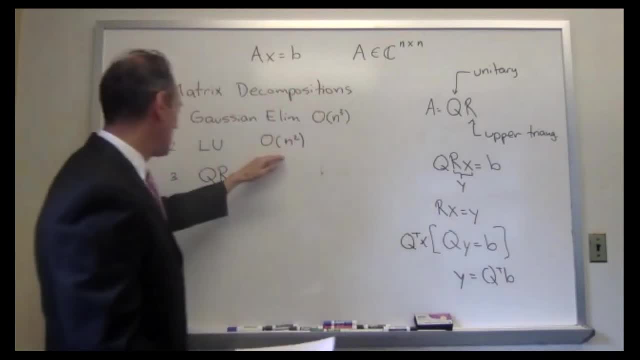 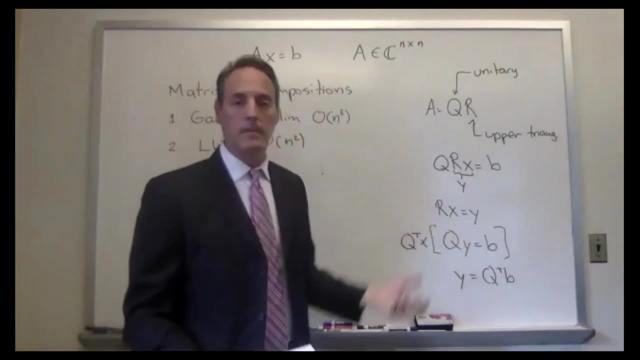 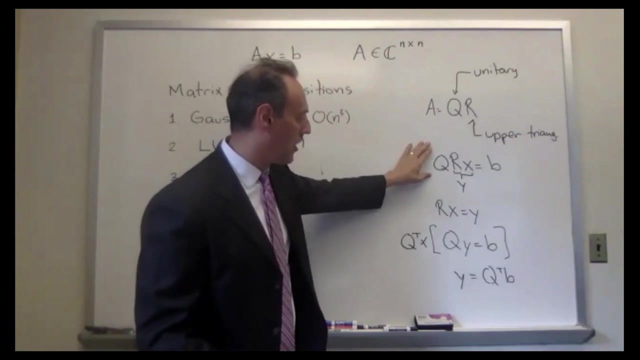 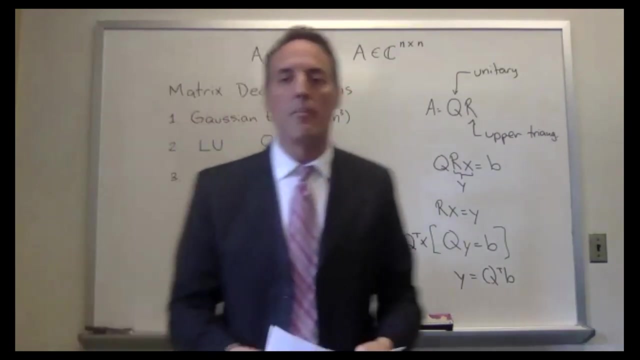 substitution. so very just like lu is going to be an order n squared operation, because i have to do this back substitution here. okay, so that's why you might use something like this qr decomposition. it has orthogonal, orthogonal vectors here. upper triangular there allows you to set up simpler systems to solve much more efficiently computationally. 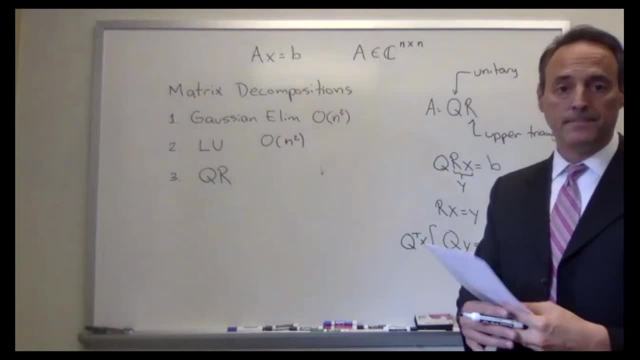 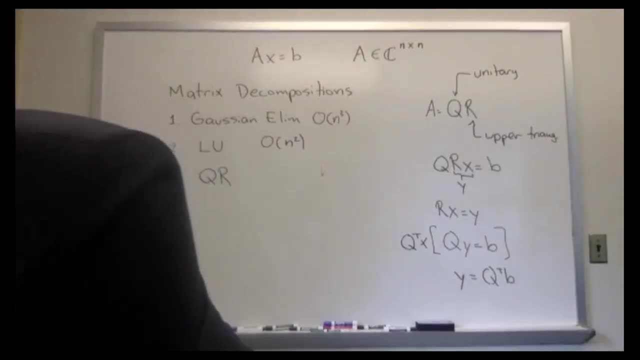 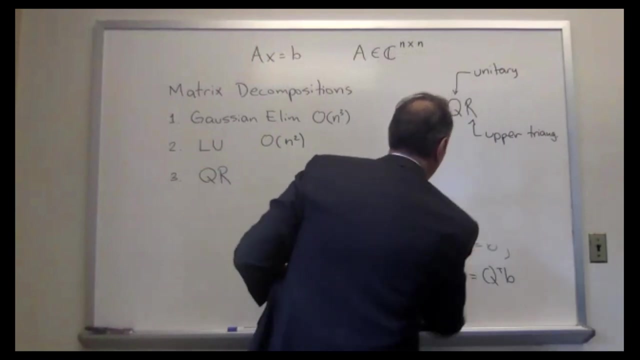 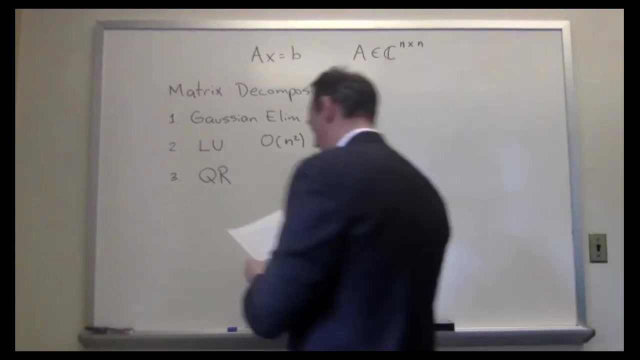 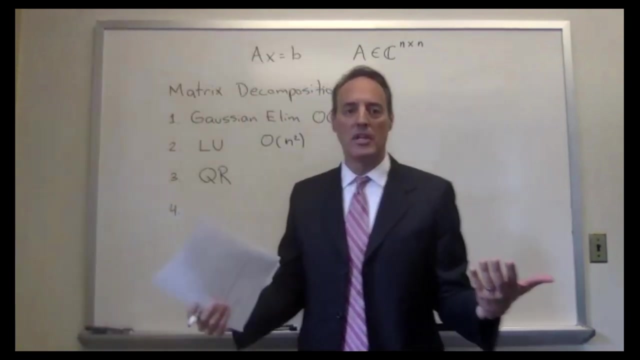 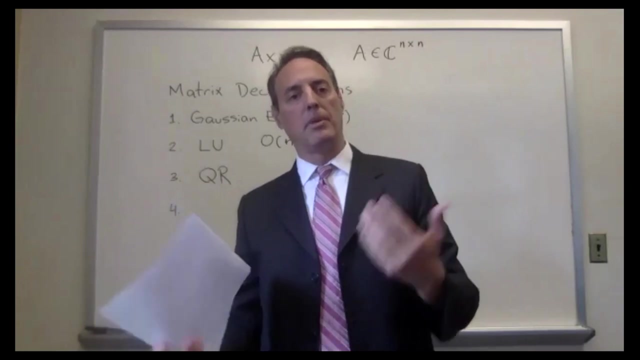 okay, good, so there's another decomposition. let's keep going, all right. so the fourth decomposition we're going to talk about- and this is one that i think everybody kind of knows- it's the eigenvalue decomposition. we uh often that's the one thing we learn in linear algebra, beyond just saying you know. 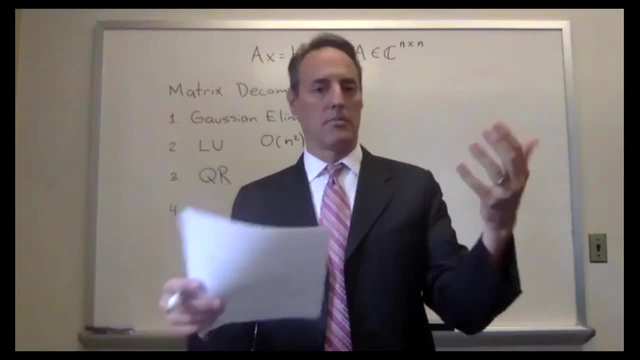 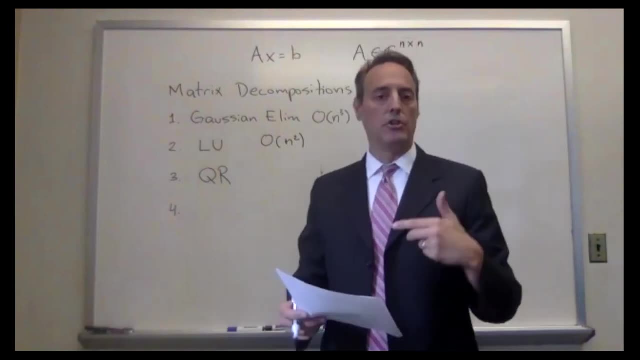 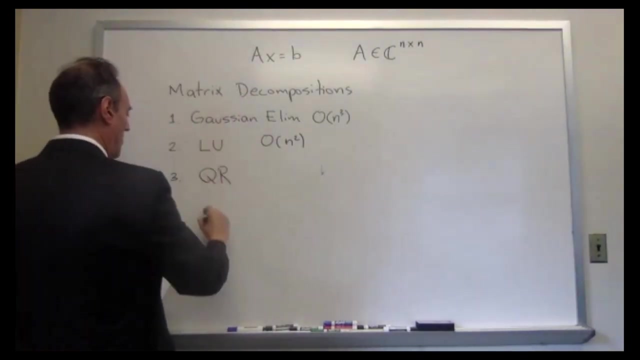 ax equal to b and do galaxy elimination. learn some things about matrices and then you might find some eigenvectors in eigenvalues. so the question is: how can you use those to your advantage in solving x equal to b? well, remember the eigenvalue problem associated with that is. 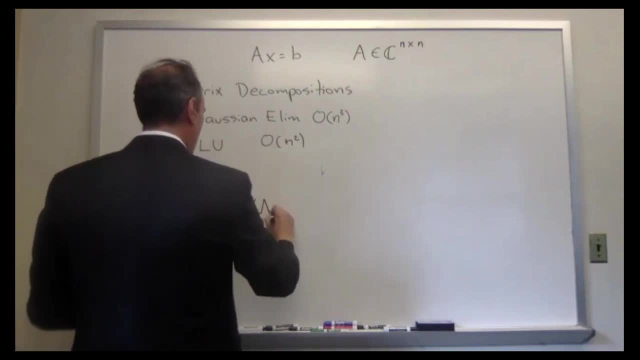 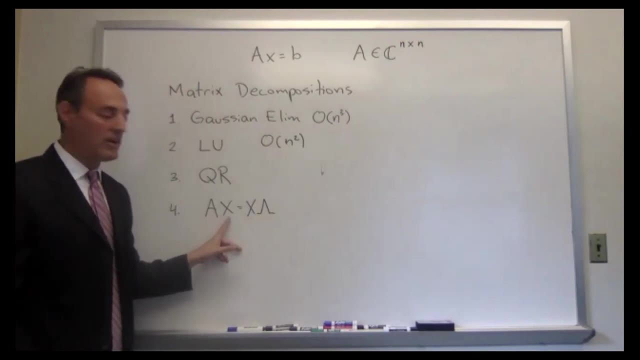 ax equals something like this: this: So I take that matrix A, the columns of x are eigenvectors and this matrix here is a diagonal matrix with the eigenvalues. This is the eigenvalue problem associated with this. So these are all the eigenvectors, all the eigenvalues. The important thing about 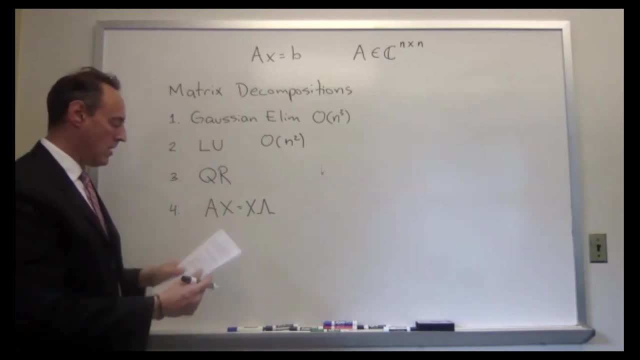 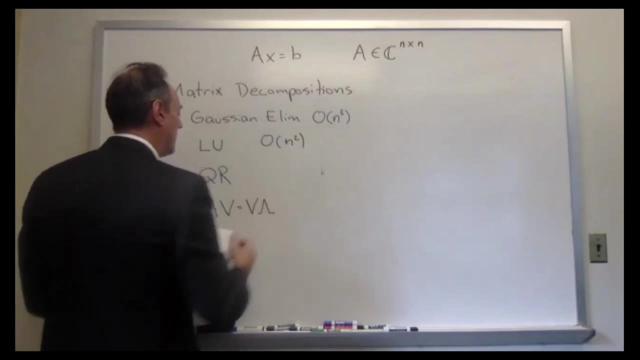 this. uh, oh, actually, let me stay consistent with my notes. sorry, I'm going to call these eigenvectors. I'm going to call them B instead A B. so B's are the eigenvectors. those are. 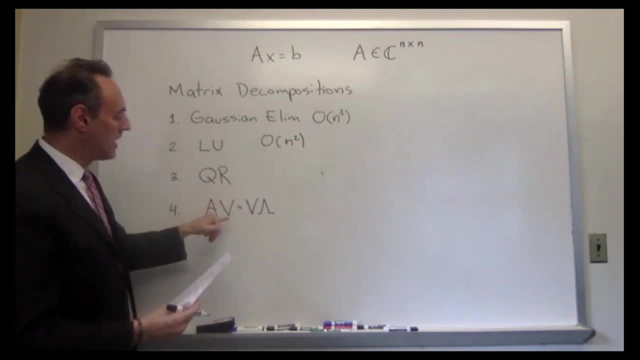 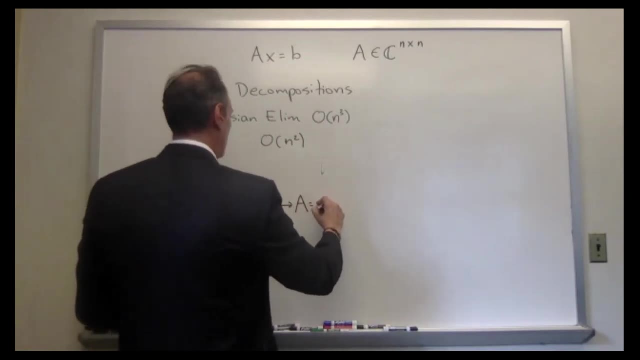 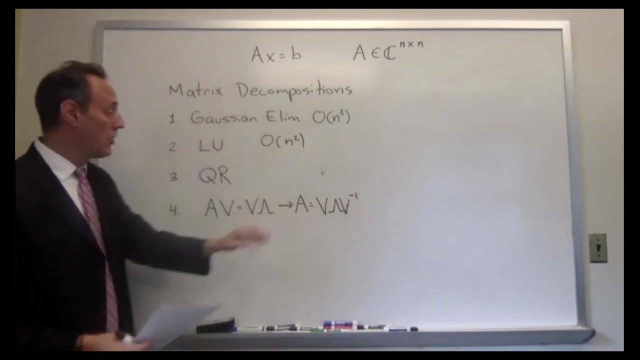 the eigenvalues. What I'm going to do is multiply both sides by the inverse of B. So what this tells you is that A is equal to. that's the decomposition. Notice the difference: L? U is two matrices, Q, R is two matrices, and now this eigenvalue is going to be equal to. 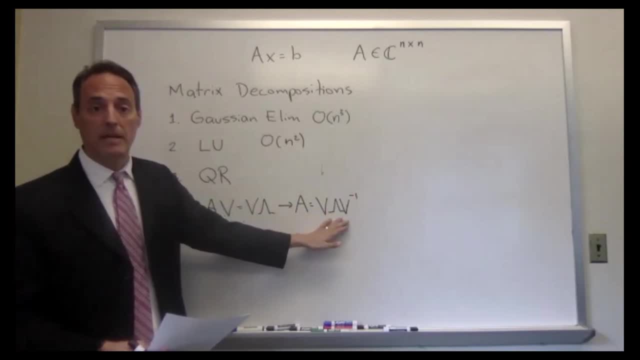 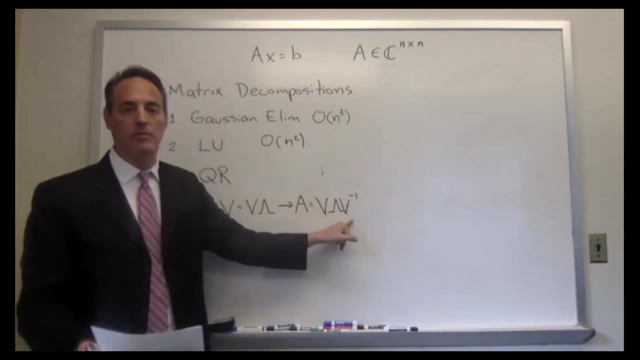 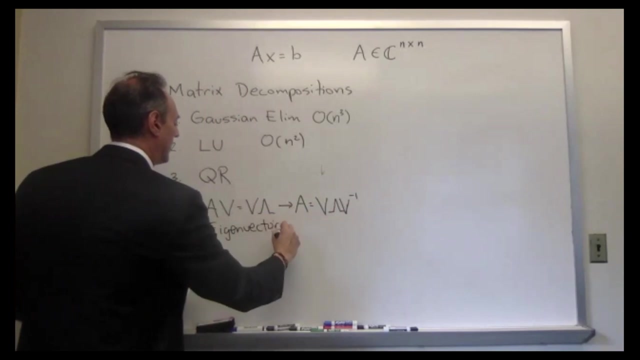 the eigenvalue decomposition. It's breaking it down into three matrices. Now notice that two of them are the same. right V is, V is there, but you're seeing B and its inverse, both here. So this is your eigenvalues, eigenvector decomposition or eigendecomposition. okay, So how could we? 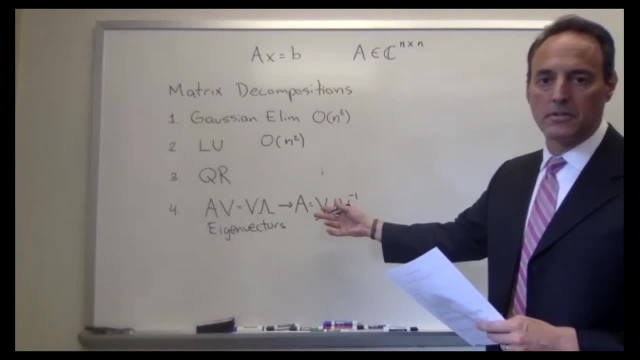 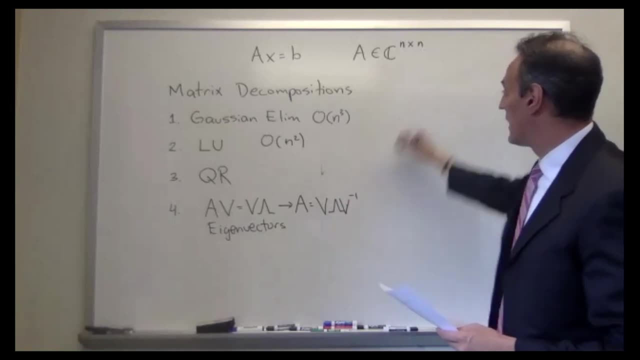 exploit the eigenvalues and eigenvectors to do this decomposition. Well, let's go back to the eigenvectors. Let's go back to AX equal to B. So A now is this guy. So you have AX equals to B, but A now is V B. okay, 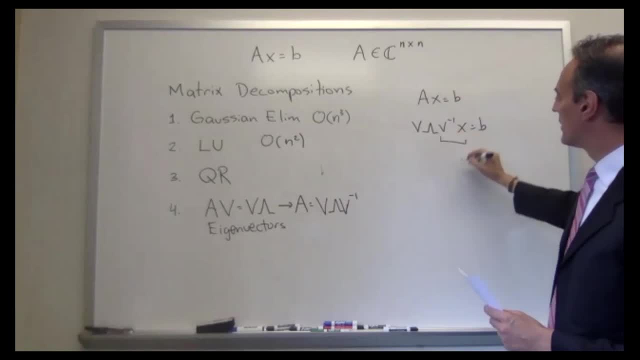 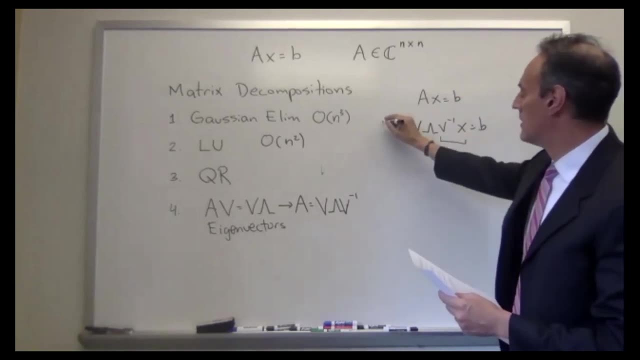 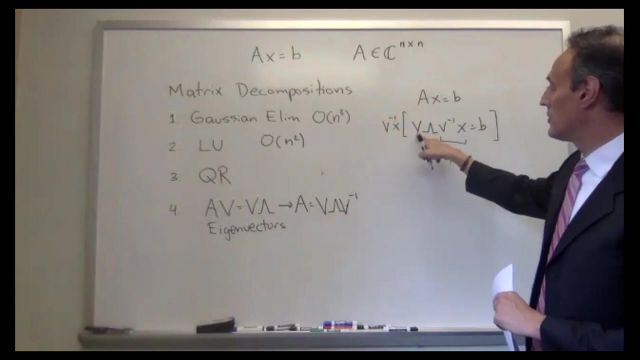 And so what you could say is: hey, how about if I call this thing here, uh, Y? and what you could do is multiply both sides by V inverse, So V inverse V identity, and then you get V inverse B. Let's call that B hat or B. 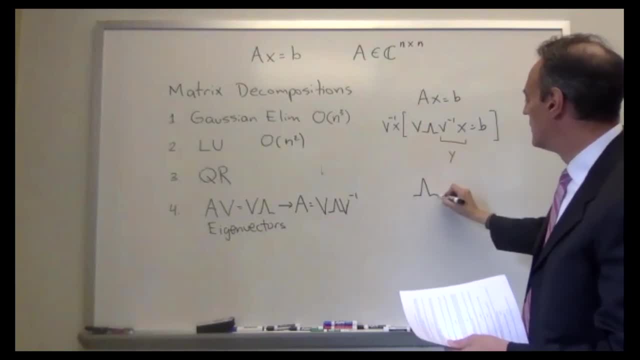 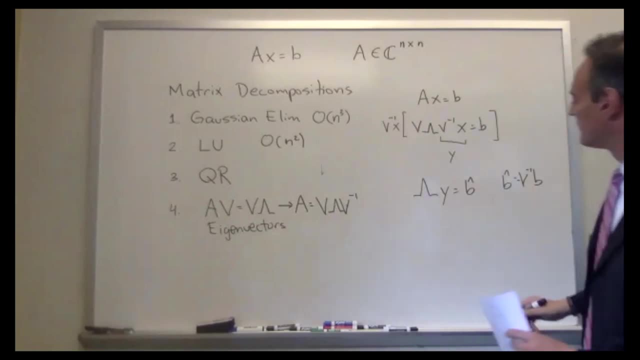 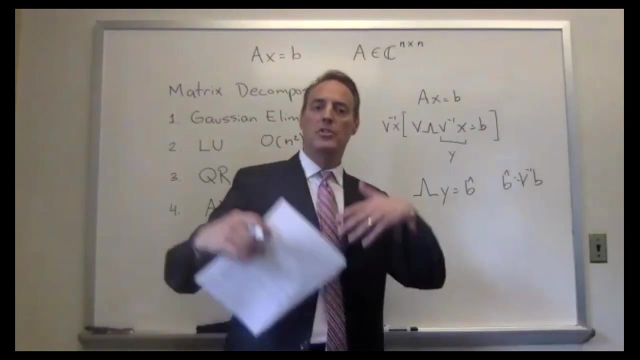 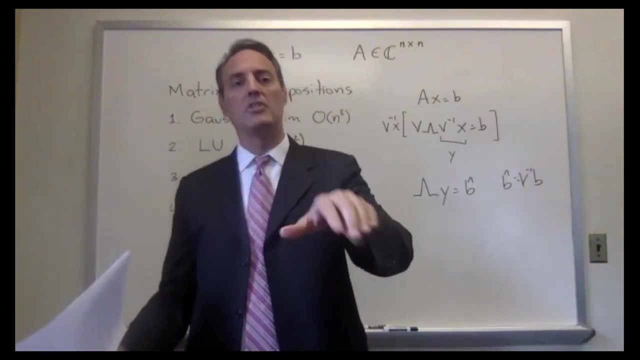 hat. yeah, So then what you would end up with is where this B hat is V inverse B. So what I've done is: I've made a transformation, I've moved into eigenvector coordinates by making this transformation. and you ask the question: what advantage did I get by doing that? 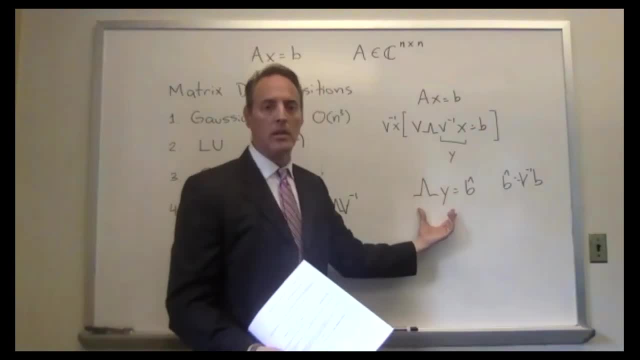 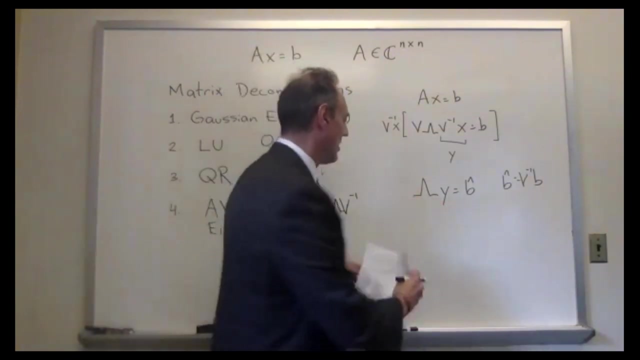 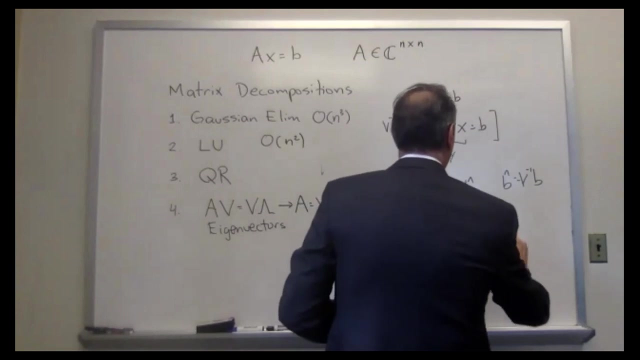 What I got is a new linear system of equations. But here's the awesome thing about this linear system of equations: What did I say this matrix was? It was a diagonal matrix with the eigenvalues. This is already solved. then It's in diagonal form. In other words, you know, this thing here is lambda one, lambda two times Y. one Y two. 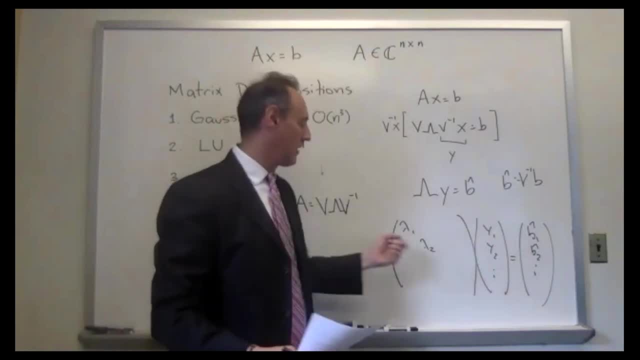 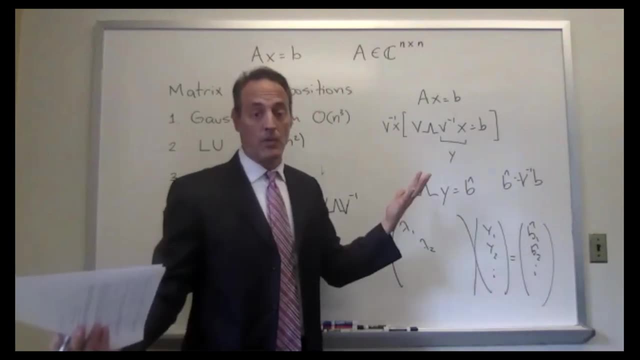 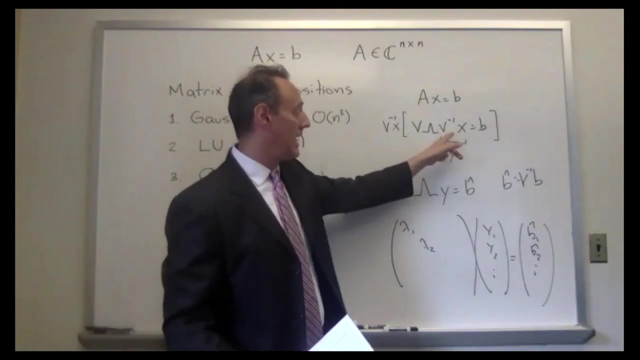 So Y one is equal to B one hat divided by lambda one. Y two is B two hat divided by lambda two. I've got it all solved, Okay, And once I get this Y right, Then I can- just I can- get back to X by multiplying by V. 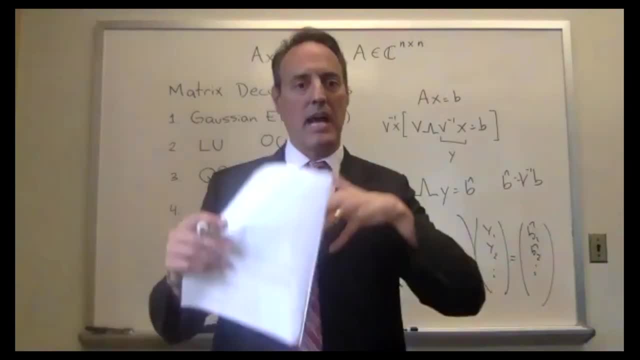 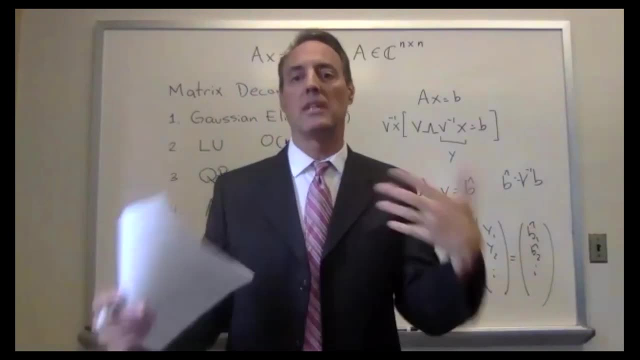 So the beauty of diagonalization is I actually just solved the problem already. I put it in this form where it's. I get the entire solution out, just because it's in diagonal form. By the way, for those of you guys with the physics background, 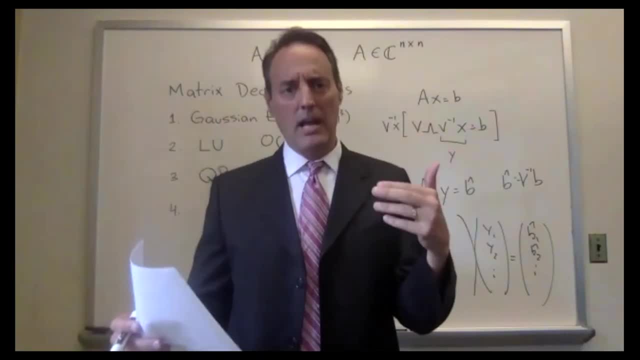 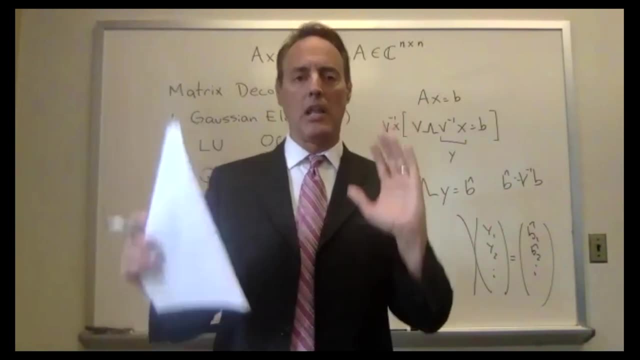 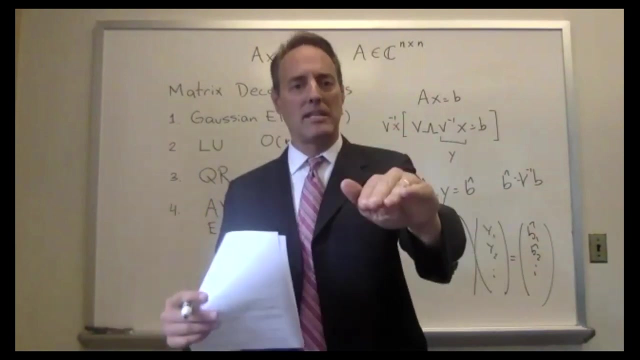 Also in an engineering background. You know one of things that eigenvectors are always used for. this is why every people really know eigenvectors or experienced them in the past, is because a lot of these physical systems, which one of the most important coordinate transformations to make is- to put it in a 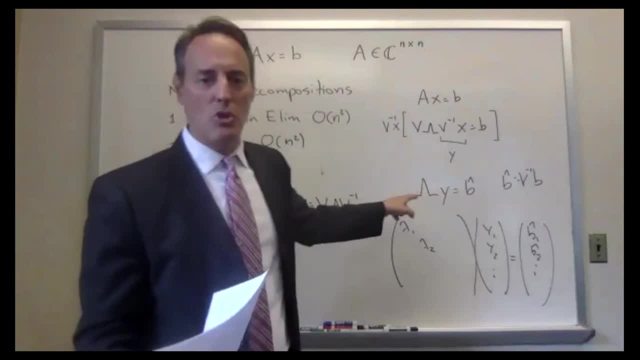 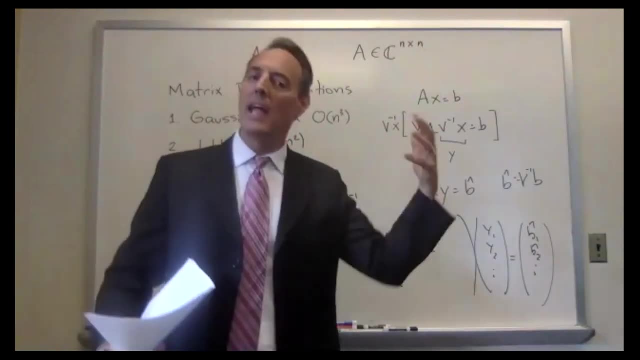 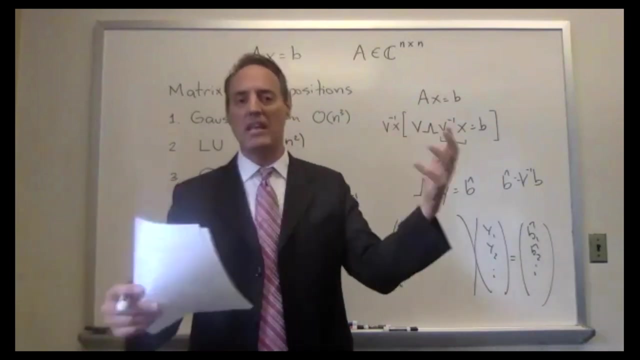 diagonal framework. i just showed you how that works. i just i made a transformation to a new variable y and in this new variable y, everything's diagonal, everything's easy. instead of n equations with n unknowns that are all coupled, it's n equations that are one by ones. 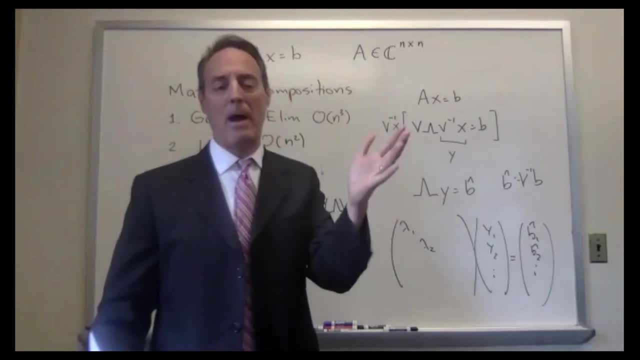 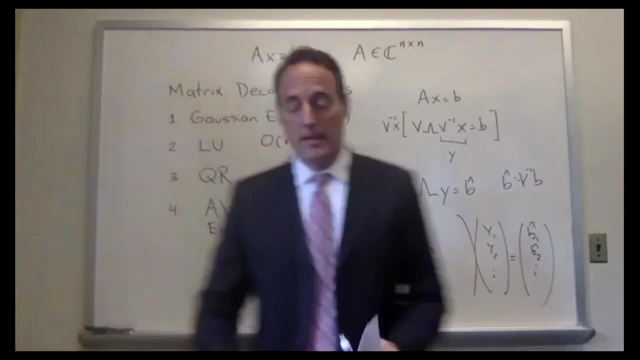 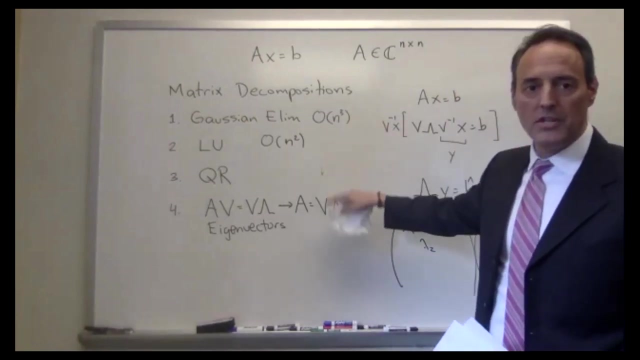 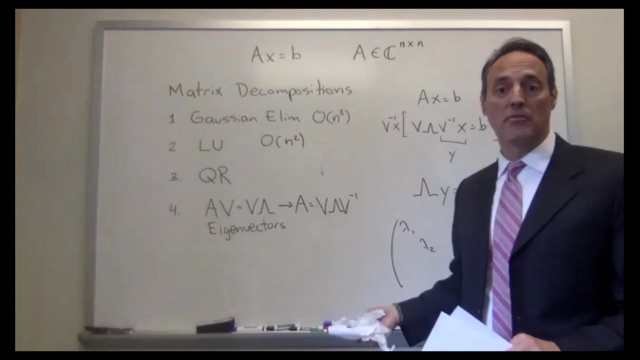 that's. that's the power of eigen decomposition. okay, so that's one possibility. now, uh, one of the things we're going to be talking about throughout is there's different reasons you'd use these. eigen decompositions are fantastic. you can't always produce an eigen decomposition of a matrix. 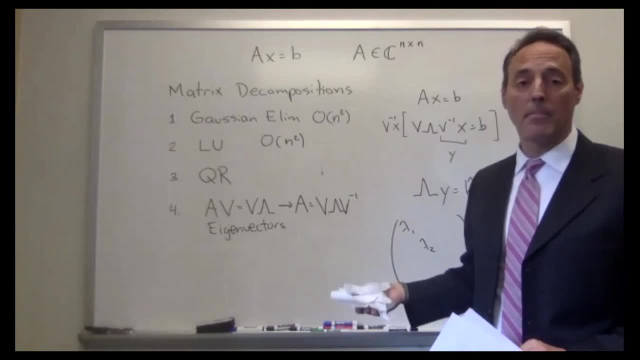 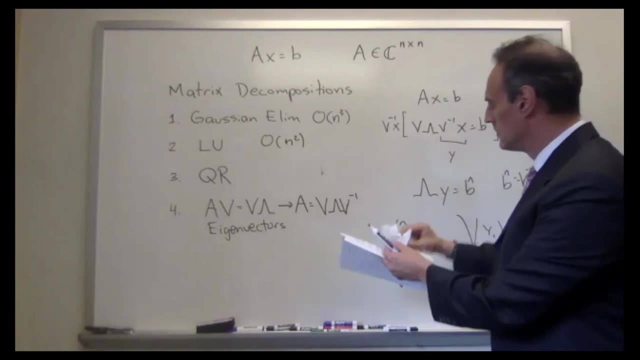 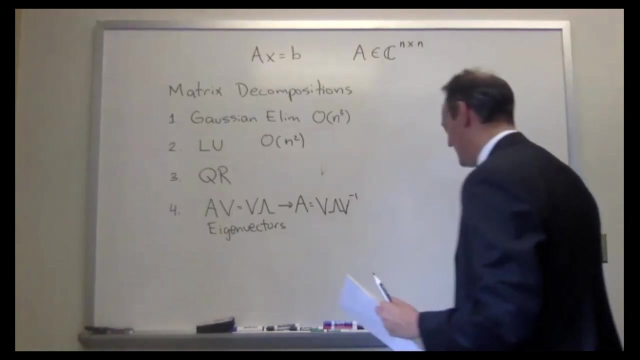 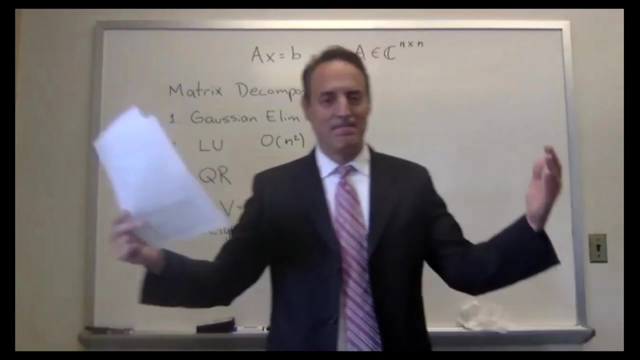 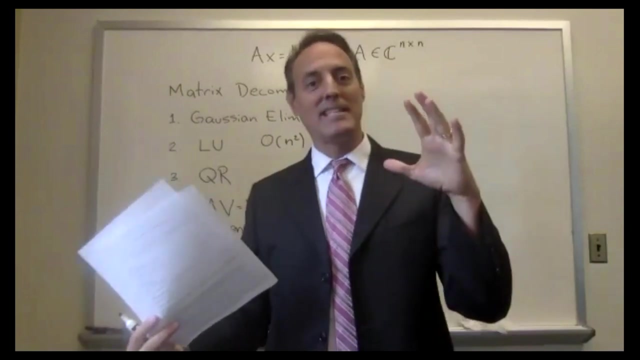 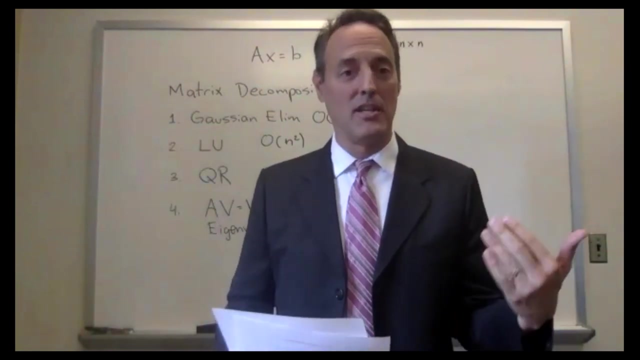 it's not guaranteed to happen. you have to have certain properties of a matrix to do it, okay. so just keep that in mind. that that's the concept here. all right, next decomposition: you know how thor has his hammer? well, anyway, this is- uh, this is the molnier moment. like we're gonna pull this. this is the svd. 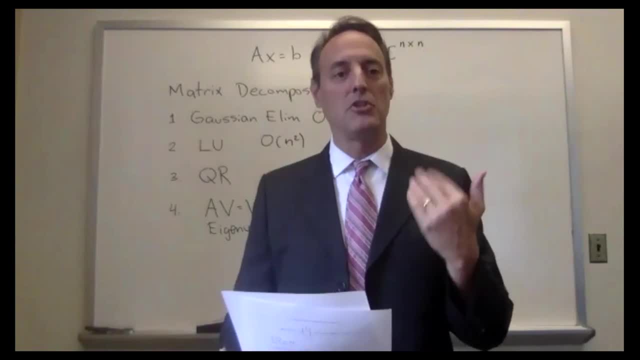 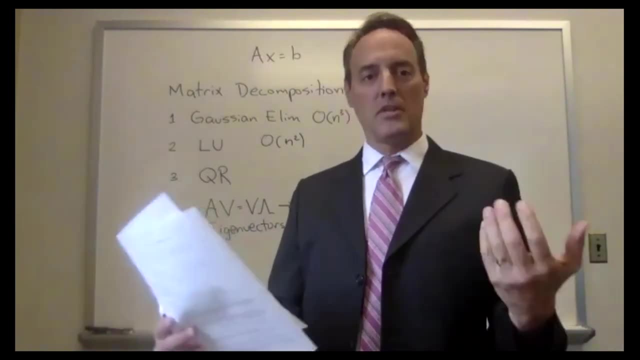 the singular value decomposition. in my view this is the most important decomposition you need to know. i am a little bit surprised that when you come out of a lot of linear alphabet courses in undergrad you've never heard of it. i never did. but to me the singular value decomposition is one of the most. 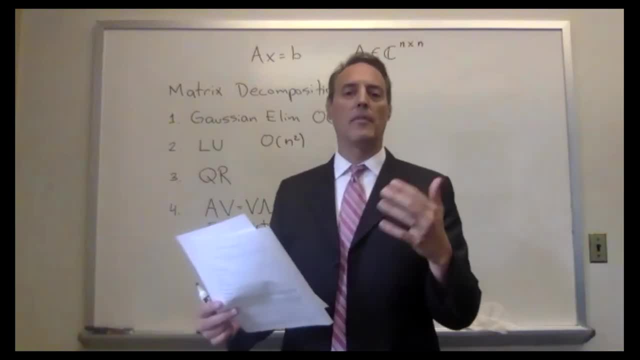 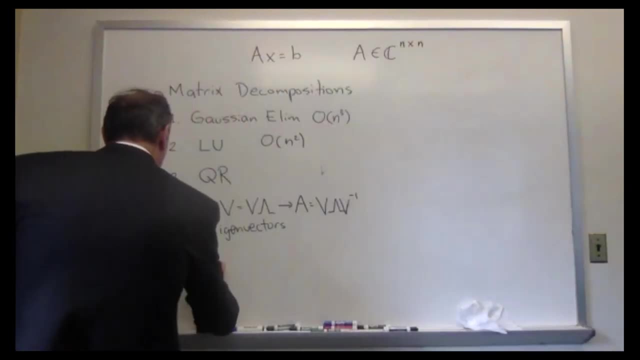 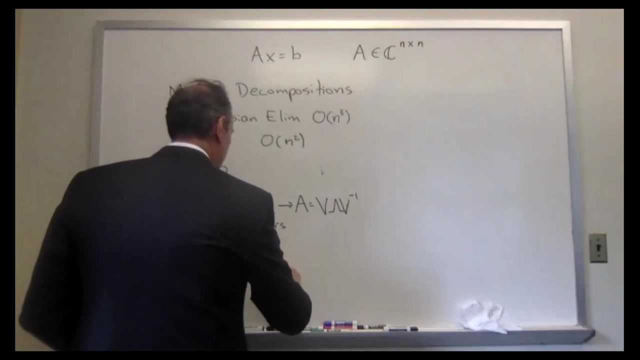 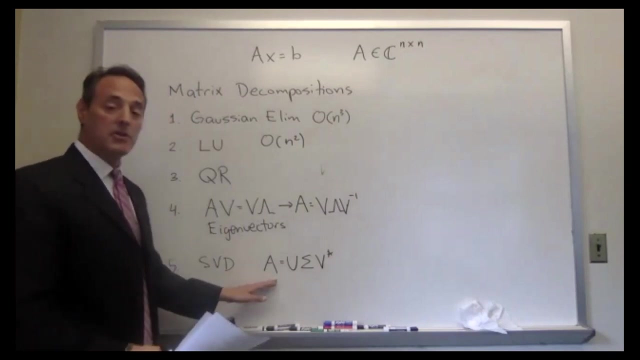 powerful. it's one of the ones that is, frankly, what is so powerful and so effective in terms of the. if you're going to pick one decomposition to know it's the spd, so spd- singular value decomposition and it's a product. it breaks the matrix up into a product of. 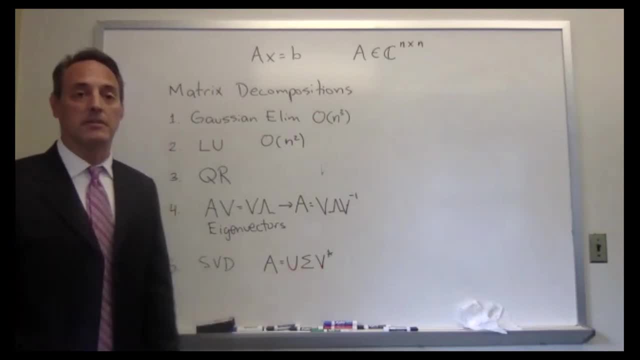 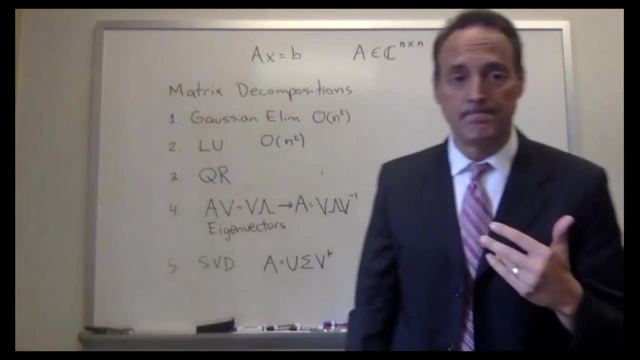 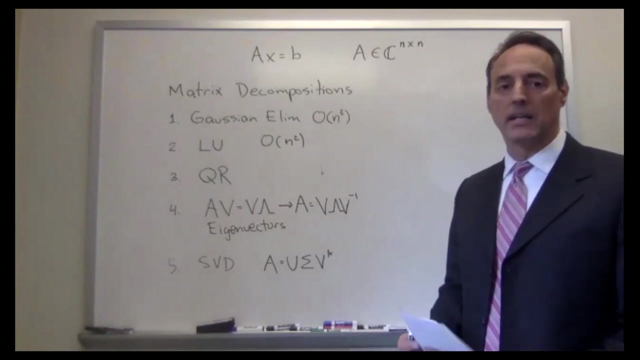 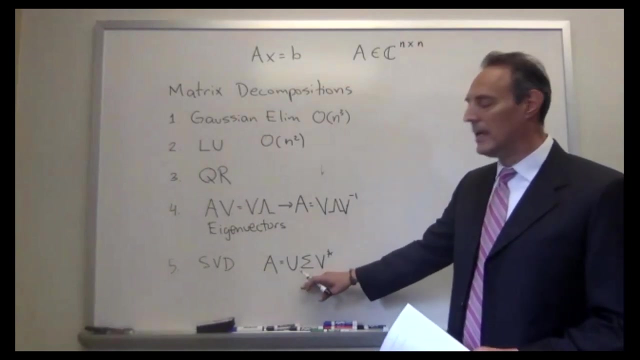 two unitary matrices and a diagonal matrix. okay, we're going to spend all next week talking about spd. it's one of the workhorse decomposition algorithms that people come up with. it's fantastic. it really is an amazing. uh, it's an amazing decomposition. notice how close these are to each other. 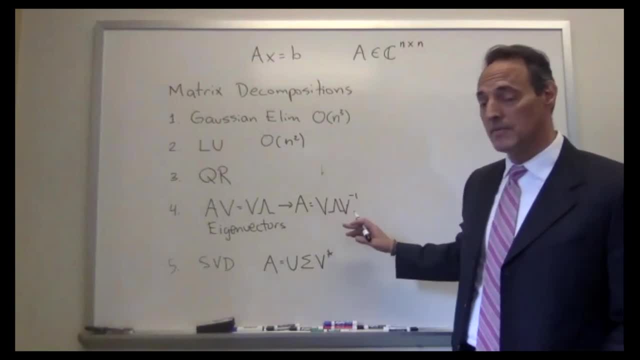 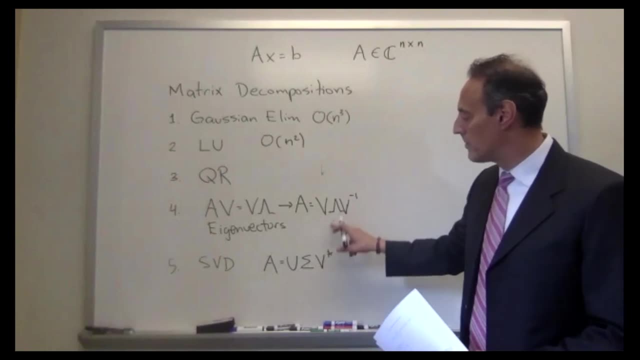 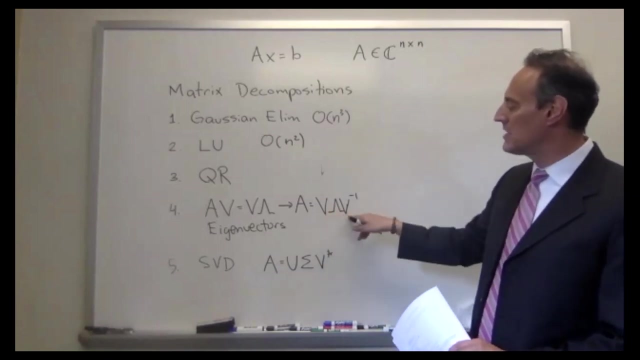 we're in fact make connections between eigen decompositions and spd. the identity composition and spd looks similar, right, look three matrices, three matrices. the middle is diagonal. but here's the power of the spd. the eigen decomposition requires one set of vectors b, which are eigenvectors here and it's inverse there. so this is. 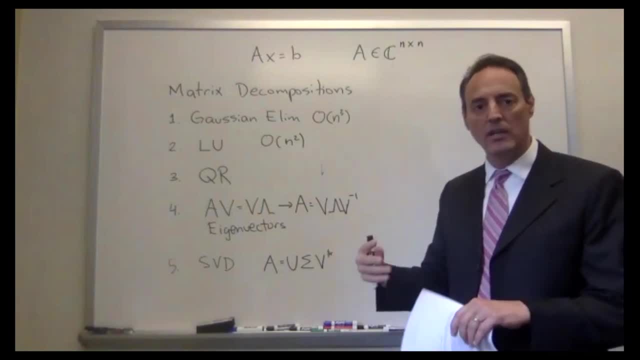 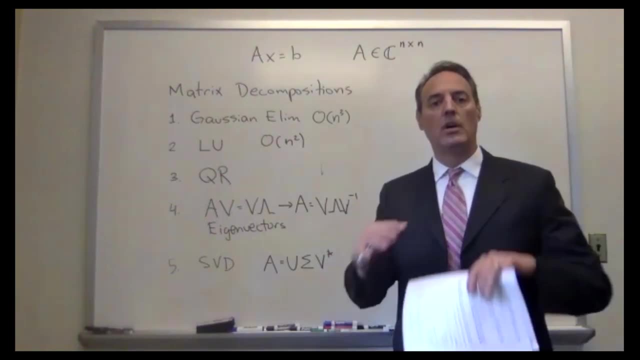 not two independent coordinate systems. it's the same one, that you see. both it and its inverse, spd, works with two orthogonal coordinates. so it's not two independent coordinate systems, it's the same one, that you see. both it and its inverse, spd works with two orthogonal coordinates. 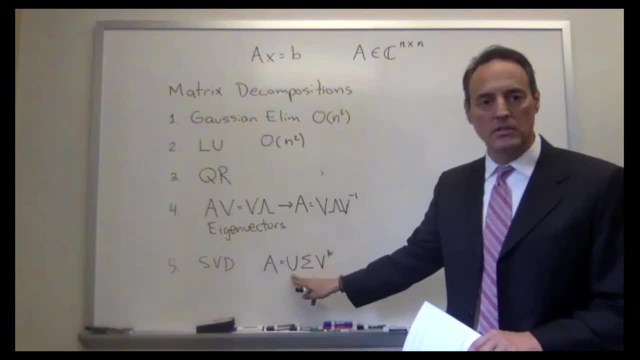 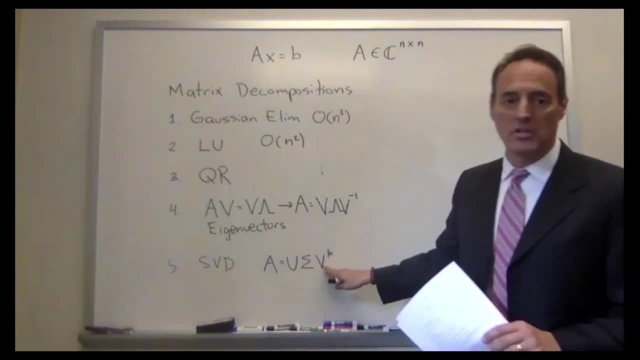 so it's not two independent coordinate systems, it's the same one. that you see, both it and its inverse, spd works with two orthogonal coordinates. right, this is a unitary matrix, which means all the columns are orthogonal unit length. this is another unitary matrix: all the columns are orthogonal unit length. 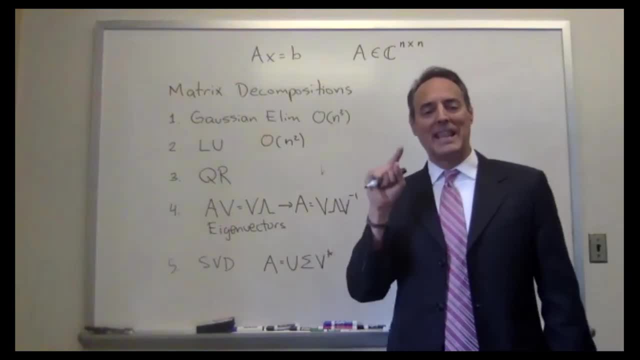 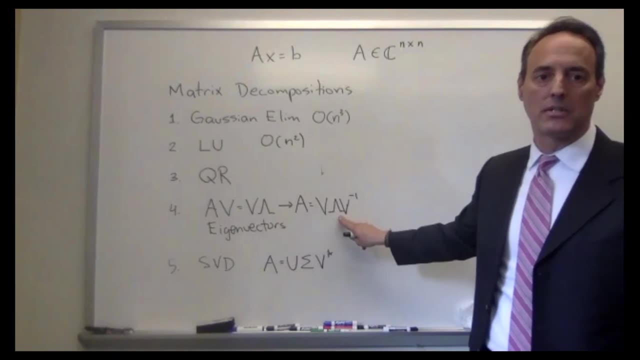 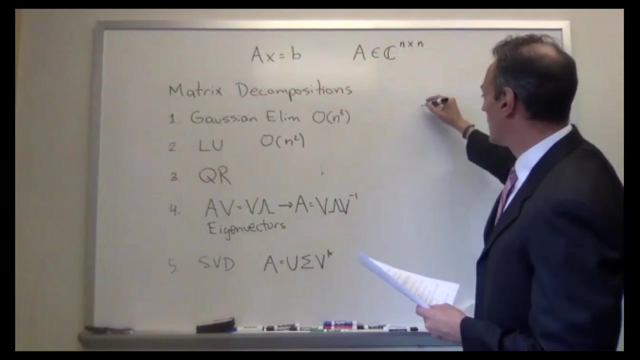 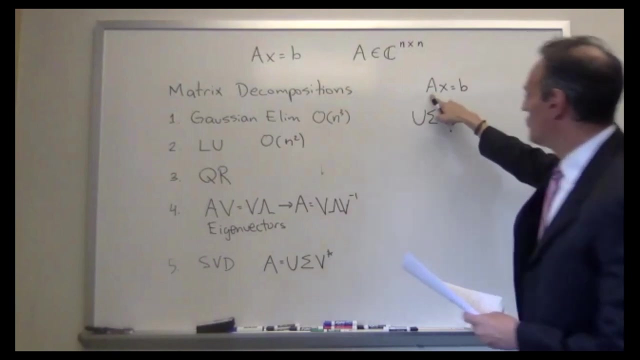 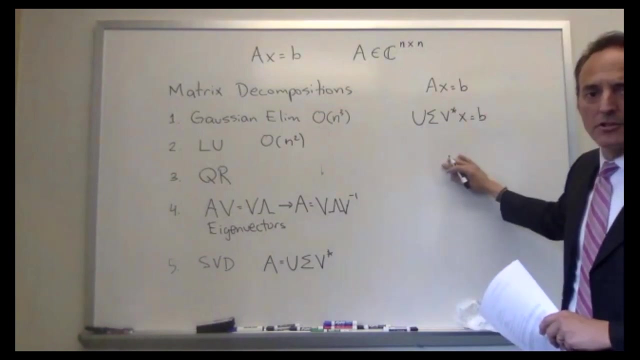 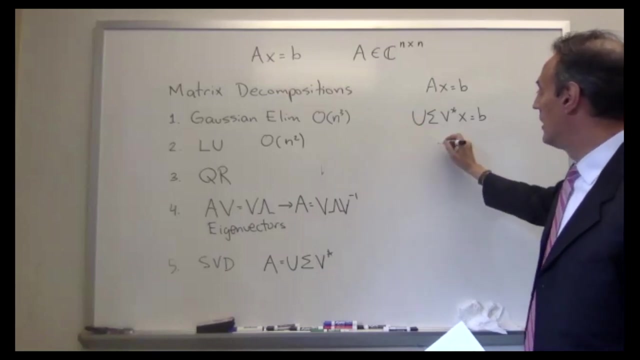 two orthogonal coordinate systems. it's that flexibility that gets you so much further than this constraint of having one coordinate system in the top right. so i thought this was. then I can just call this X hat and this B hat And notice what I've done. So this: 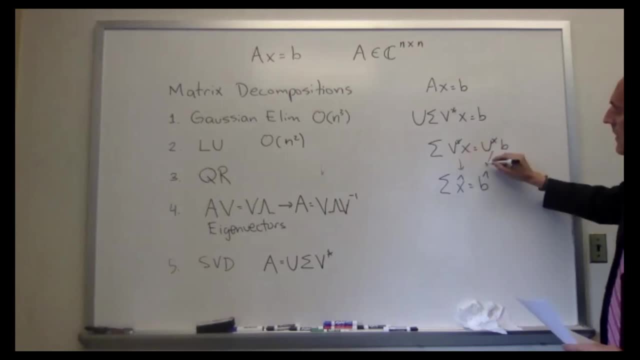 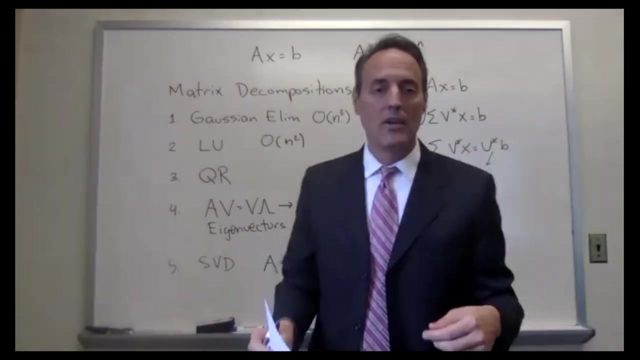 is X hat here, that's B hat here. This is now a new linear system of equations, but this matrix here is diagonal, so I get the same thing I did with the item vector decomposition. It's in diagonal form, It's n one-by-one equations. 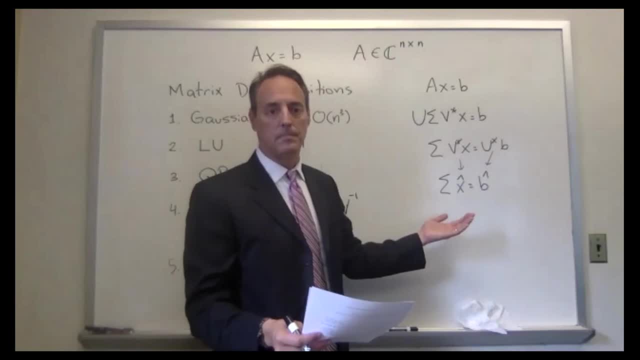 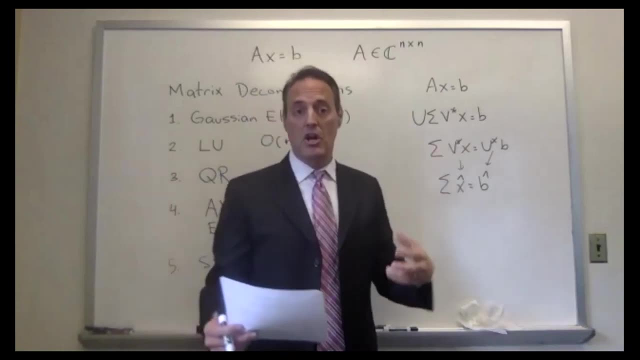 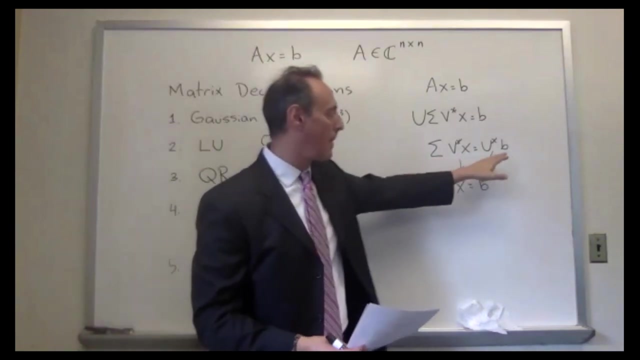 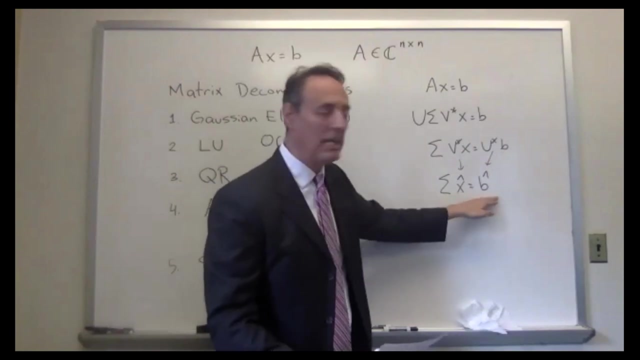 trivial to solve because it's in diagonal form, And I've moved myself into a new coordinate system where what I do is, if I have this decomposition, I project X into the V unitary matrix, I project B into the U unitary matrix to create these new embeddings called X hat, B hat. 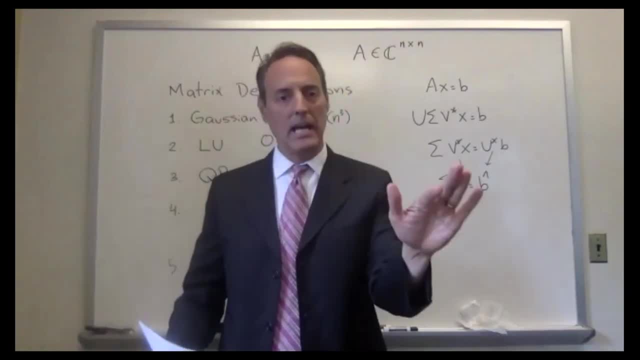 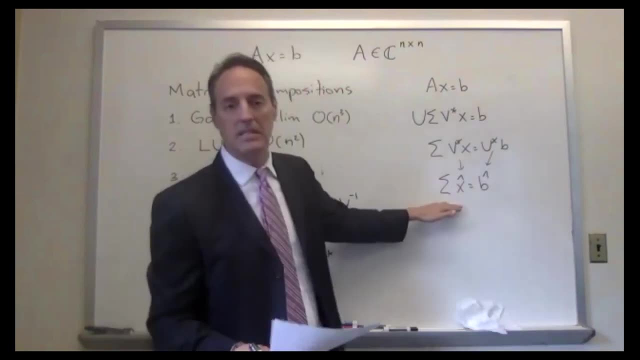 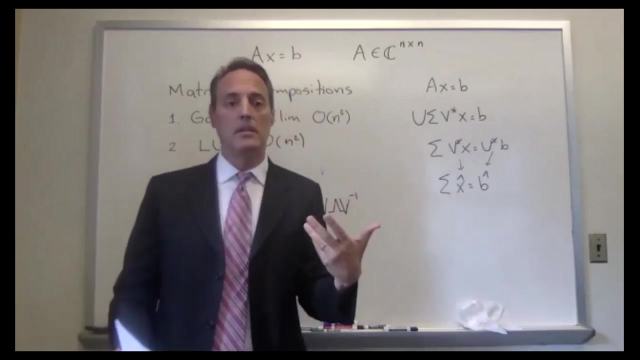 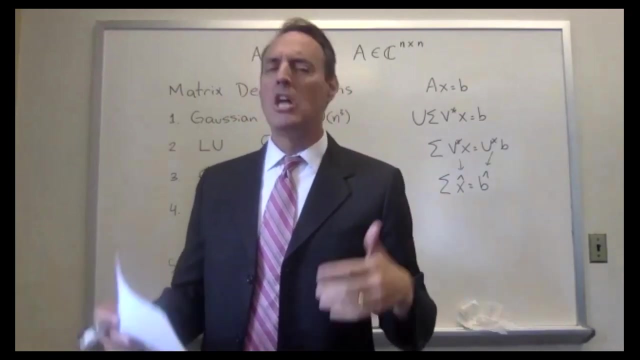 and in that coordinate system, everything's diagonalized, Everything's independent. Every direction is independent of all other directions because this is diagonal. By the way we'll go through this, I am guaranteed that the SVD will work for any matrix, Square, non-square, any matrix. 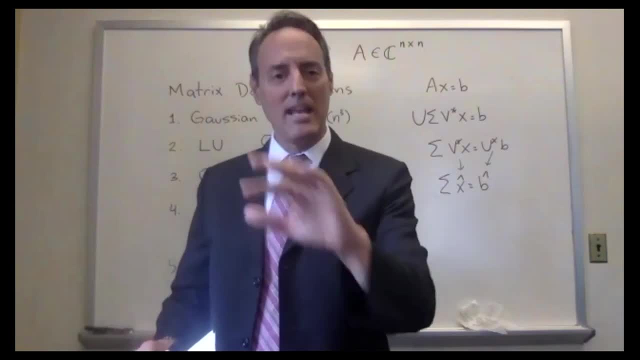 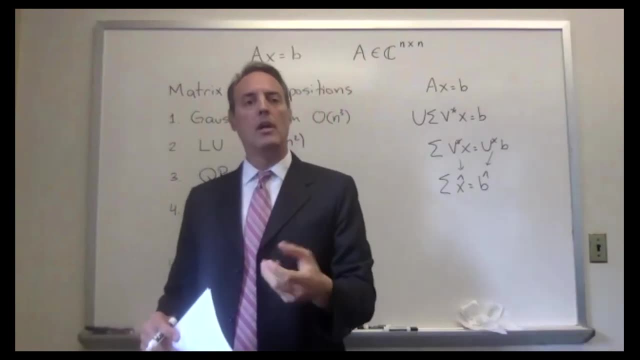 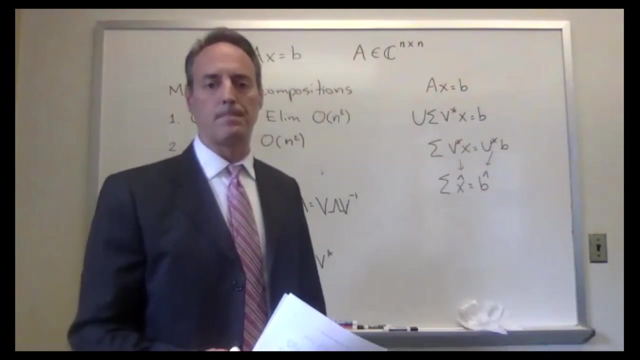 Singular complex, any matrix. Keep that in mind. Really important. Most decompositions work under certain constraints, One of the powers of the SVD. it doesn't matter, You just give me a matrix, it will have an SVD. Okay there. 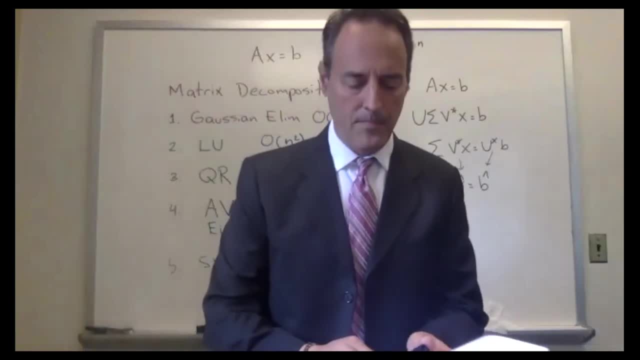 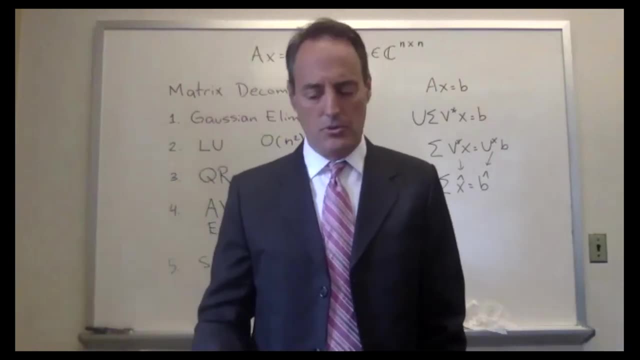 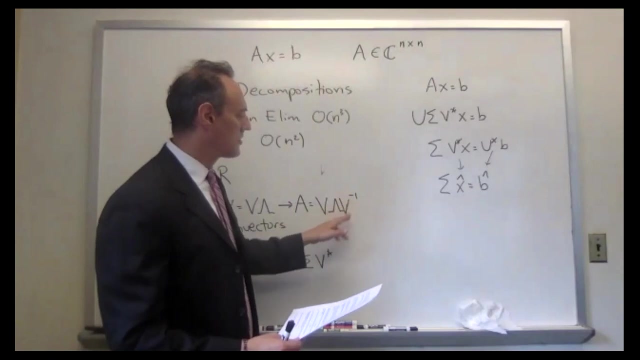 are a couple other ones, but we're kind of pretty close here to the time. One of them is called the shore decomposition, and the shore decomposition is restricted to square matrices And again it looks very similar to this, except for now, instead of the inverse, you do the transpose complex. 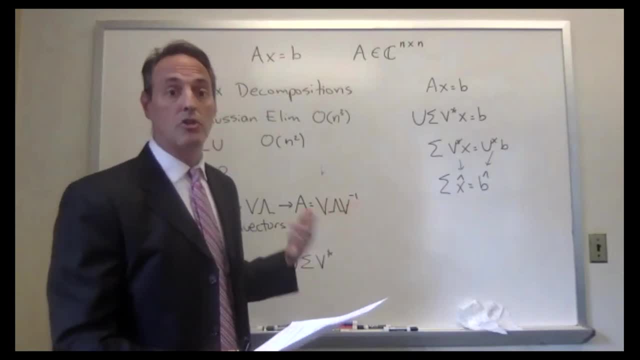 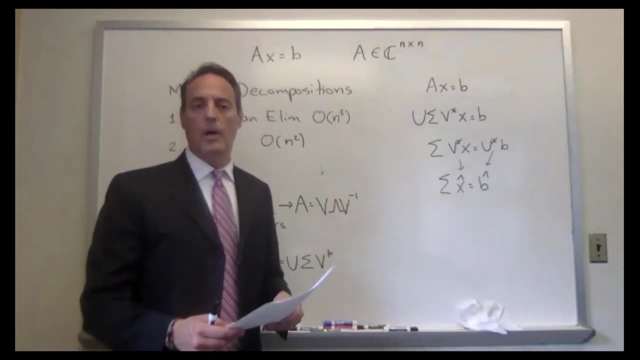 conjugate. That's the shore decomposition. You can do that decomposition as long as it's a square matrix. And the other one that I'll list here and these notes I'll send to you is called the Cholesky decomposition. The Cholesky decomposition. 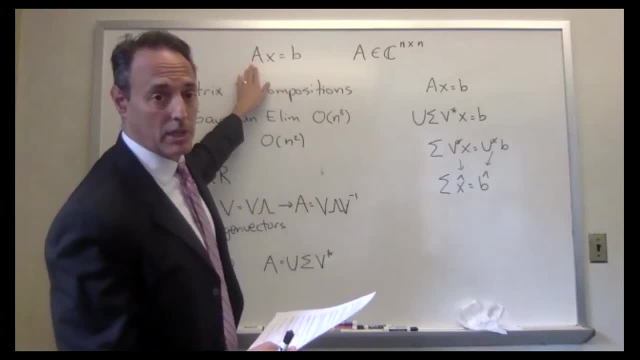 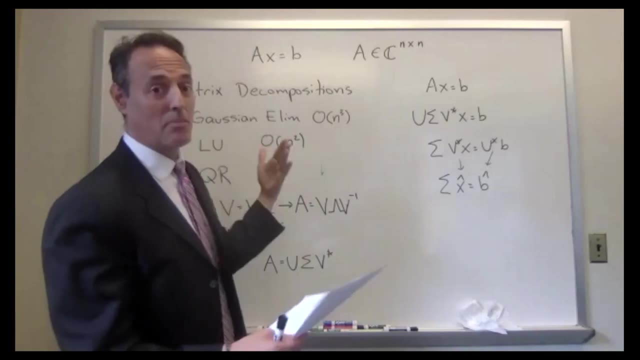 takes advantage of the fact that if A is symmetric- which is pretty harsh for restriction, by the way, right, There's not that many matrices that are square and symmetric. These are special matrices, But if it is, Cholesky is a really fast. 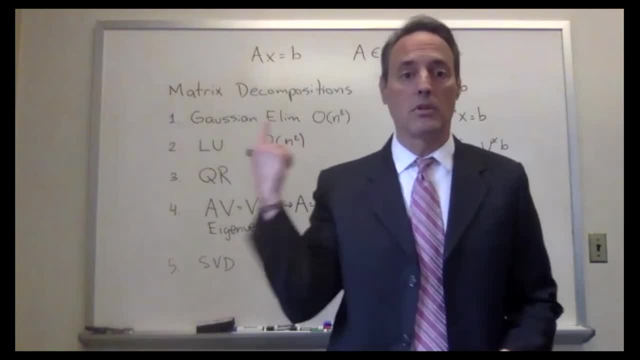 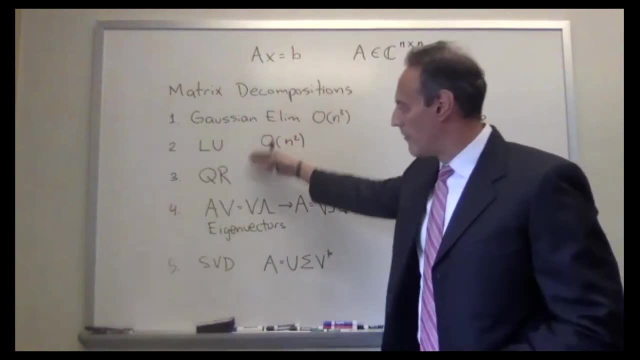 decomposition that people use to compute the solutions out of this problem, And it's again based exactly on these kind of concepts here. So you know, here's four decompositions: Gaussian elimination- again, let me just say it is not what you 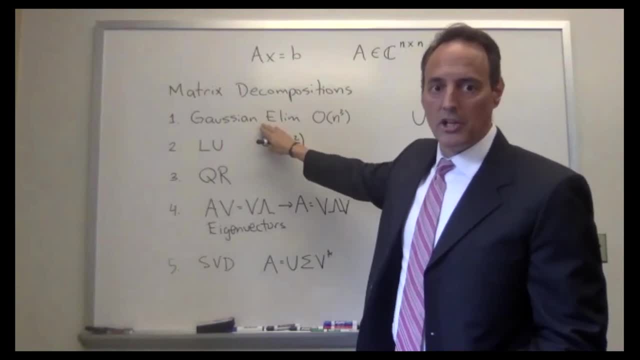 want to be doing. When you do computing, you do not want to do the slowest computational method possible. You will get fired And your science career will end and your thesis will go on forever because you're solving a linear problem. okay, for five years straight. okay, Here you're getting. 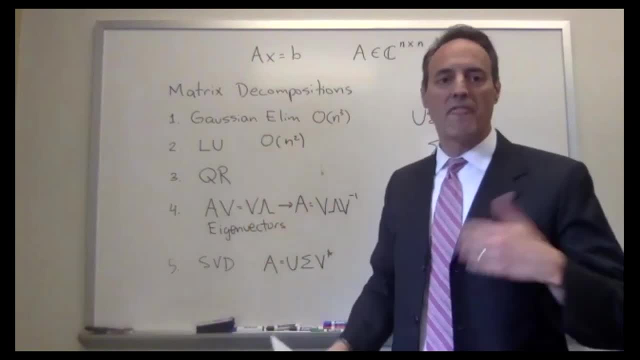 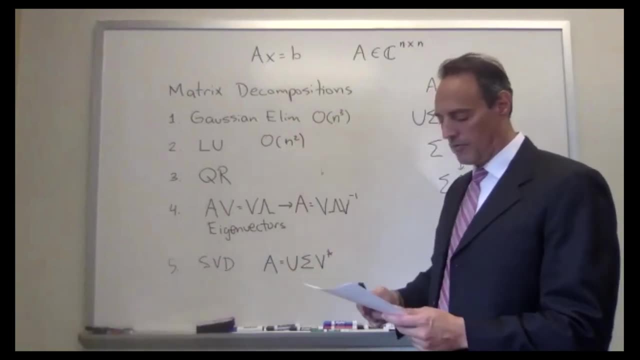 towards the power. Each one of these is built to go fast and solve things quickly and go to scale, And so there's four decompositions here. If you had shore and Cholesky, that's six. There's more. There's more decompositions, But the number of 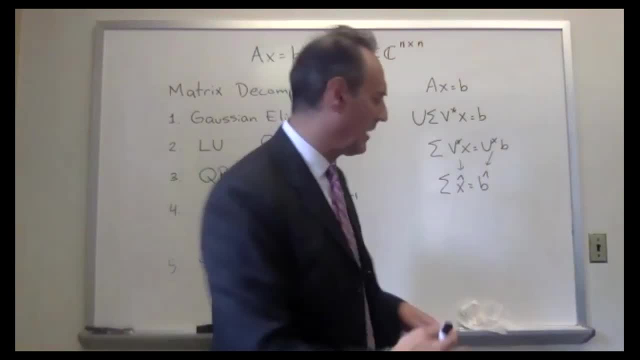 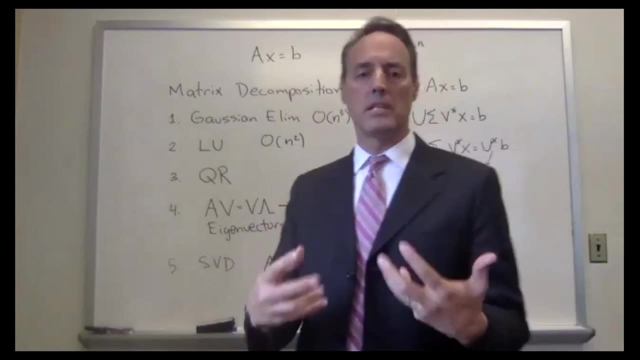 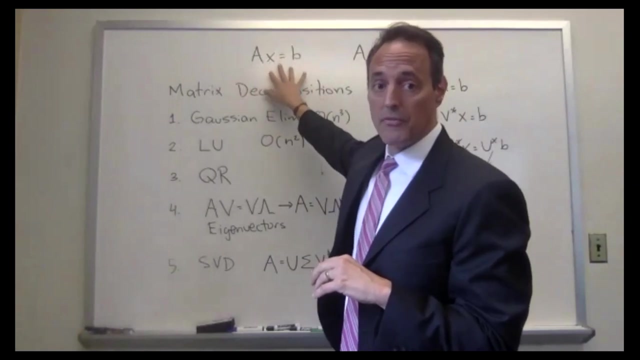 decomposition tells you a lot, because the number of decompositions is telling you that people are thinking about decomposing matrices all the time. This is what you're going to do if you're going to do scientific computing. broadly speaking, Most problems are going to come down to this, to an AX equal to B, solved. 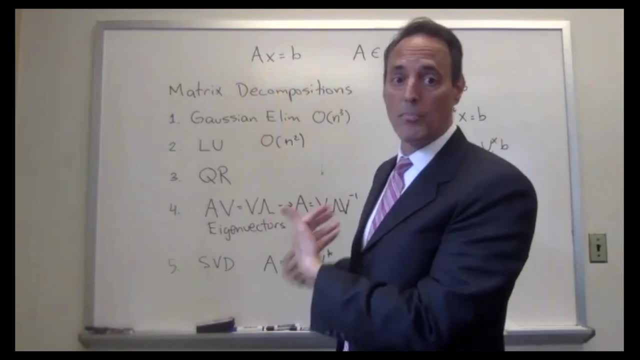 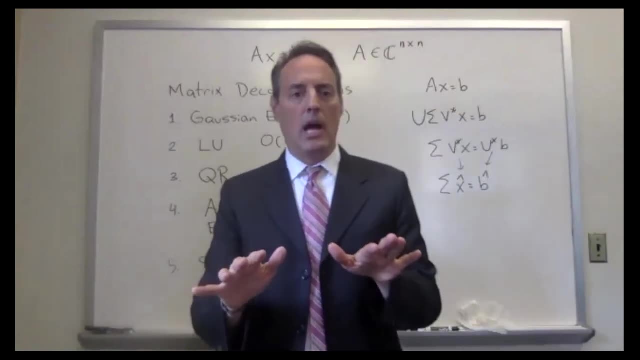 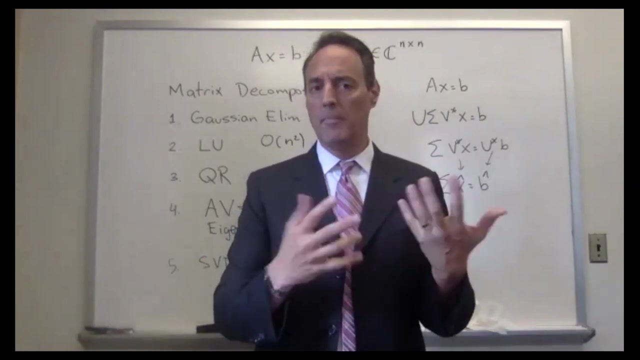 somewhere, And so it's really important to have an appropriate decomposition at your disposal to solve it quickly. That's where we're going to end. That's where we're going to end today. Let me map out what's going to happen Friday and Monday. Friday, we're going to come back to some really important linear. 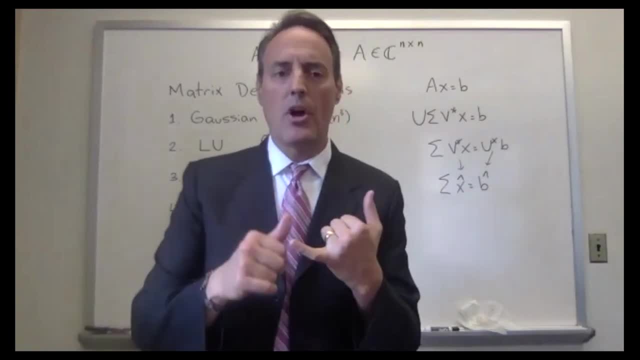 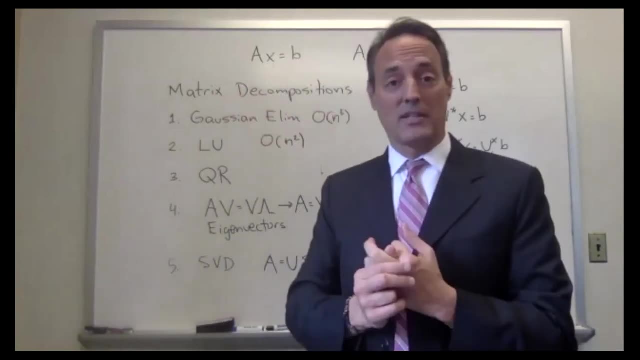 algebra concepts- They're going to be review- Concepts of orthogonality, Concepts of when can you actually solve AX equal to B? What if A is not a square matrix? Right, We got to start thinking about that, And then on Monday we're.